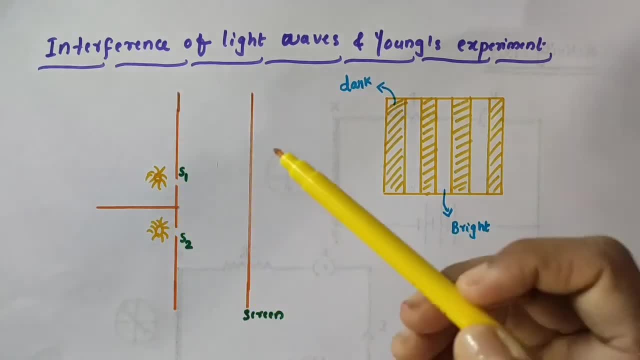 We have discussed about constructive interference and destructive interference in our previous videos. I will provide the link in the description box If you want. you can watch that. Young's experiment demonstrated the wave nature of light, and the ideas of Huggins regarding the wave nature of light were confirmed. 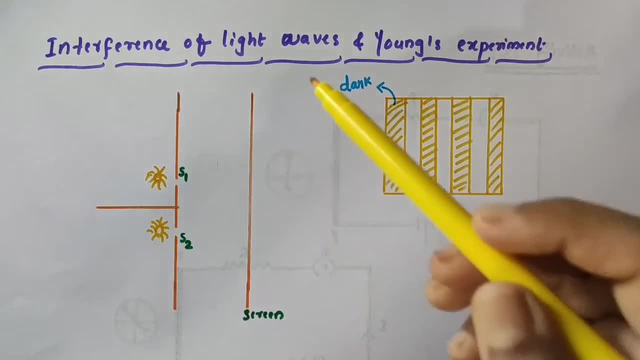 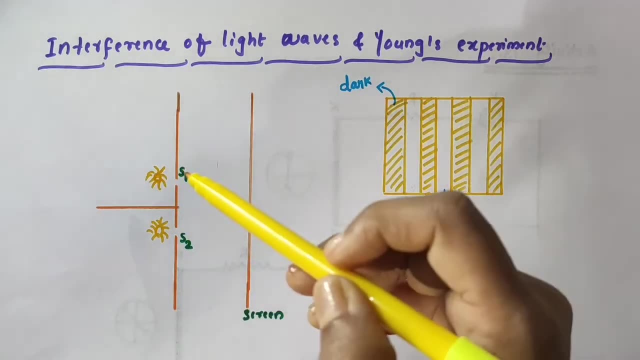 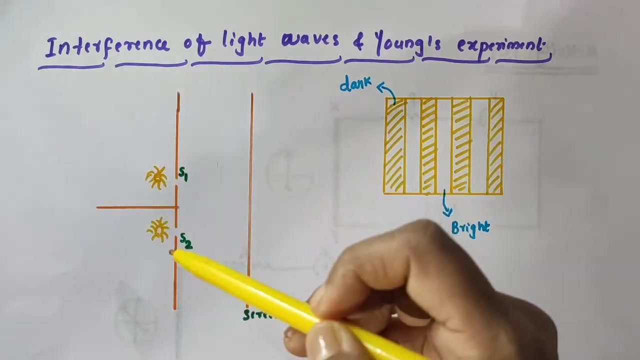 In this video we will discuss about the interference using light waves and Young's arrangement to produce interference pattern. Consider two pin holes: S1 and S2.. If we use two sodium lamps, let us assume that these two are sodium lamps. So if we use two sodium lamps, we can see that these two are sodium lamps. 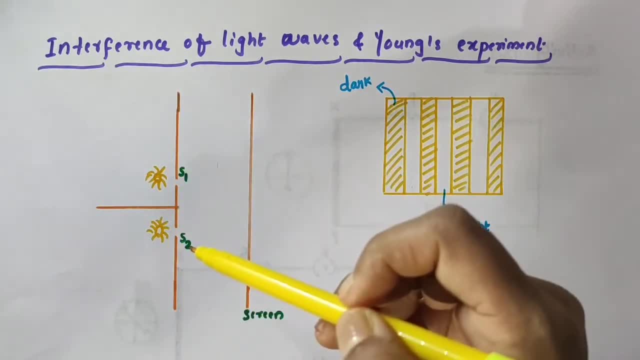 So if we use two sodium lamps, we can see that these two are sodium lamps. If we use two sodium lamps to illuminate the two pin holes, we will not observe any interference fringes on the screen. Interference fringes means the bright bands of light and the dark bands of light produced by the interference of light. 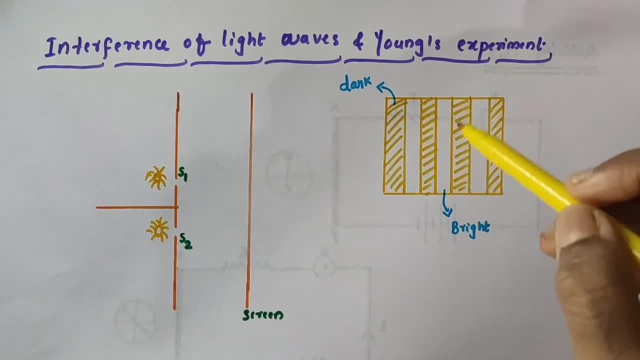 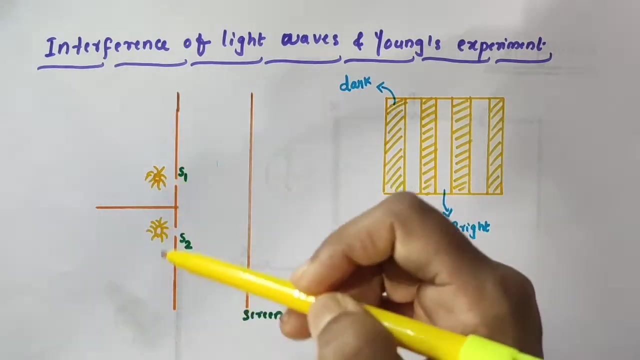 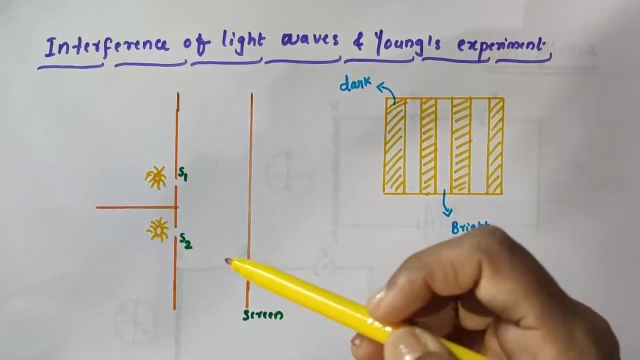 We will get a bright band of light when the two light waves are in phase, and we will get a dark band of light when the two light waves are in phase. We will get a bright band of light when the two light waves are in phase, and we will get a dark band of light when the two light waves are in phase. 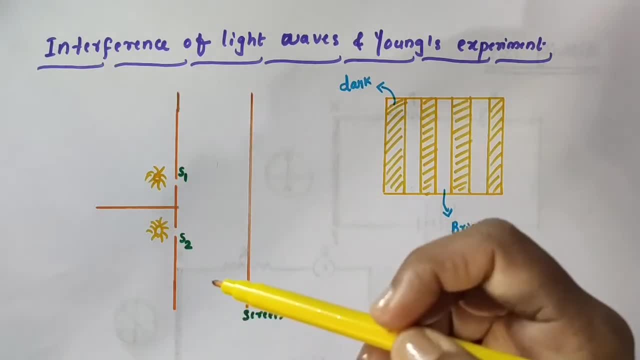 If the two sources changes rapidly with time, we say that the two sources are incoherent and when this happens, the intensities just add up, That is, the intensities on the screen will add up and no bright and dark bands of light will be observed on the screen. 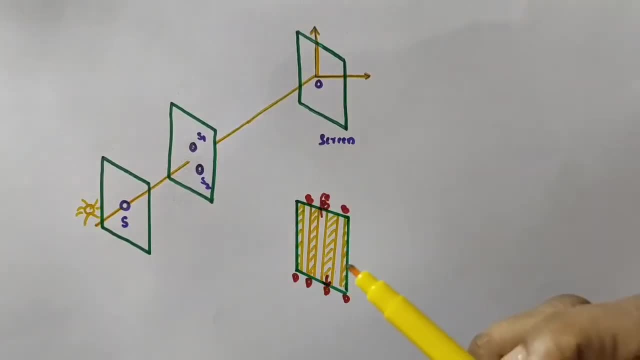 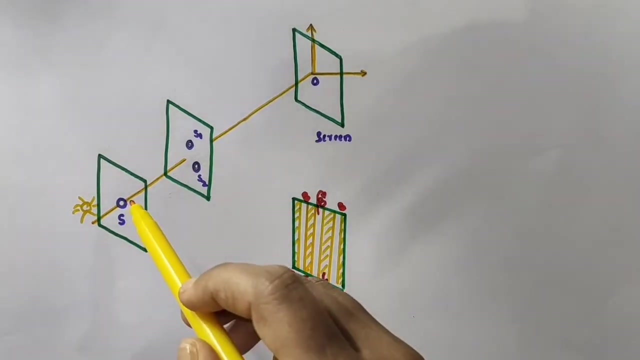 What Thomas Young, the British physicist, done was he made the two pin holes S1 and S2 on an opaque screen or an opaque object. These two holes, S1 and S2, were very close to each other. These two pinholes, S1 and S2, were illuminated by an another pinhole, S, which was in turn lit. 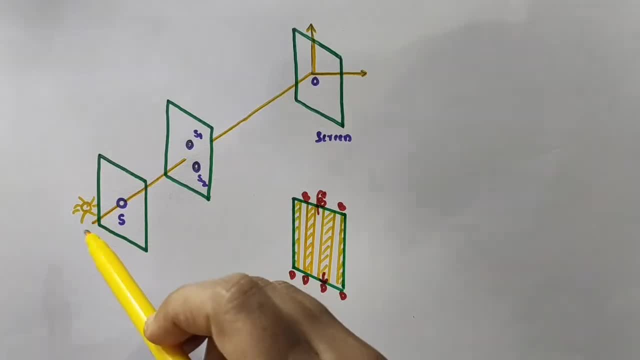 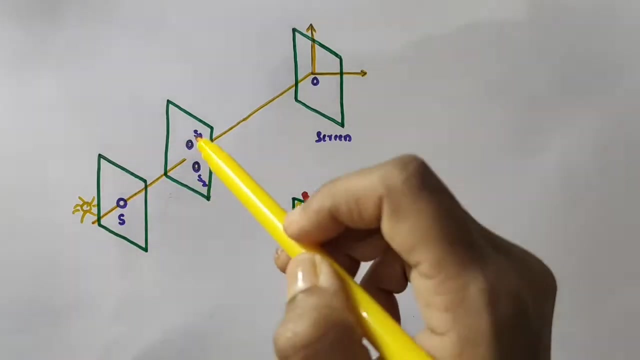 by a bright source. So consider a monochromatic light source here at S, which is kept at a considerable distance from the two slits S1 and S2.. S is equidistant from the slits S1 and S2.. S1 and S2 will behave like two coherent sources because the light waves coming 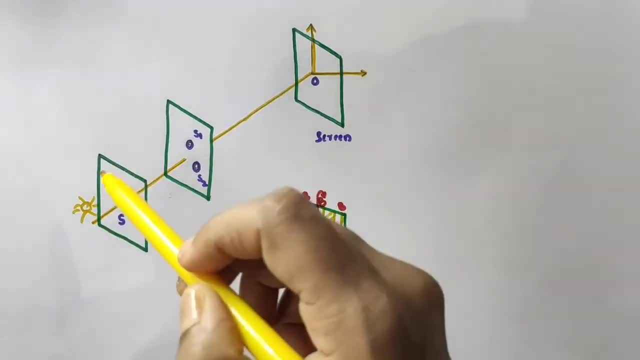 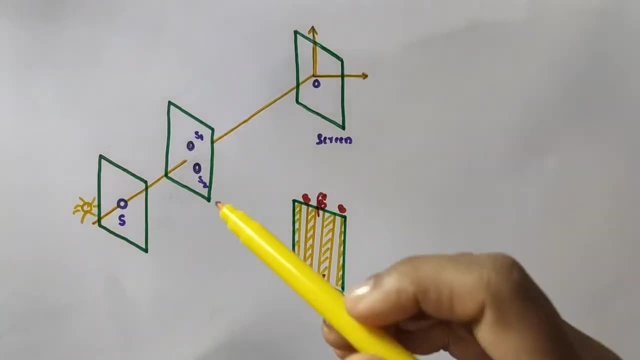 out from S1 and S2. both are derived from the same original source. Now if there is any sudden phase changes occur in the light from the source S1 and S2, then the same phase changes will be manifested in the light coming from S1 and S2.. Because 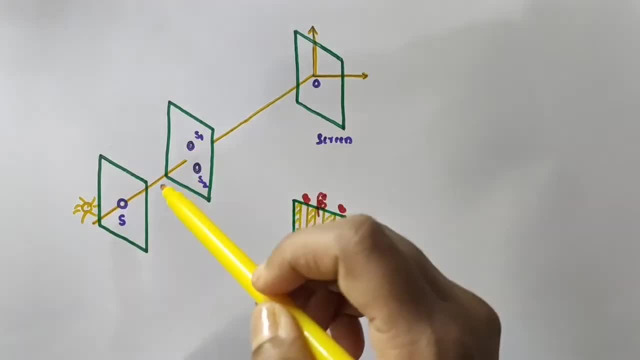 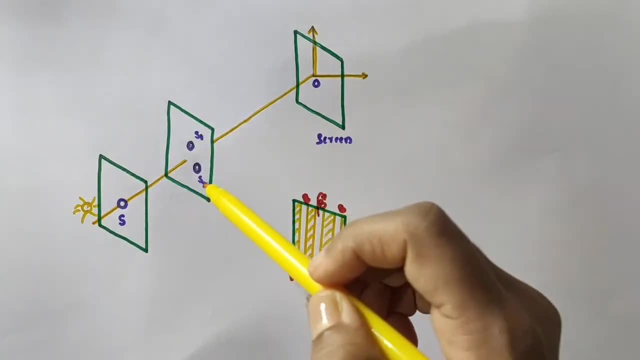 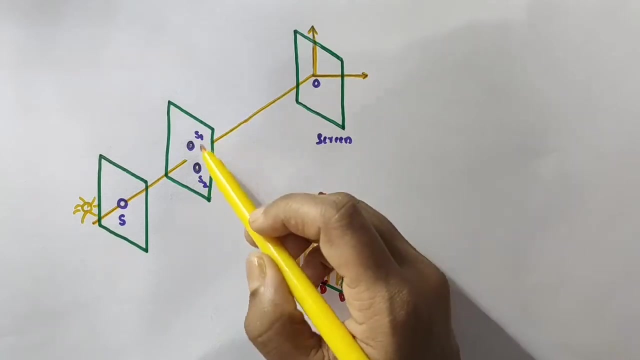 the light from S is actually passing through both S1 and S2 and they will behave like two coherent sources. So waves from S1 and S2 are in phase. Ok, now you see, when light passes through the two holes like this, we expect a bright region. 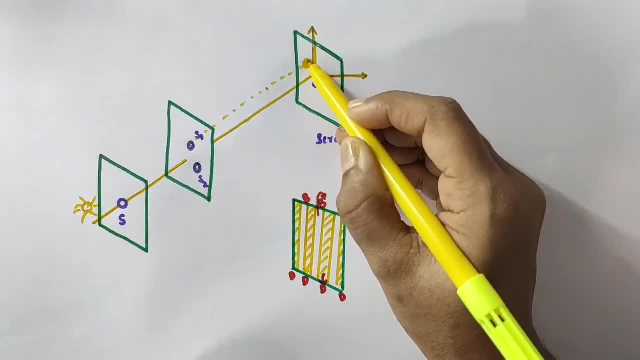 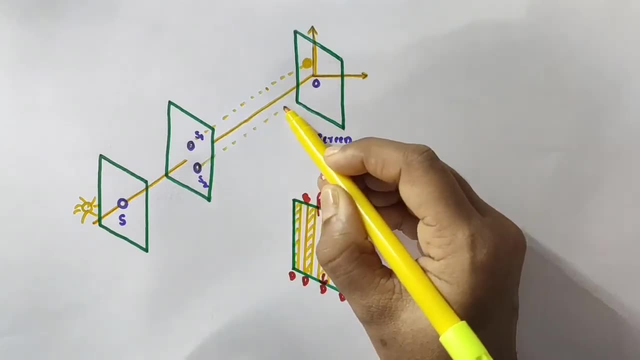 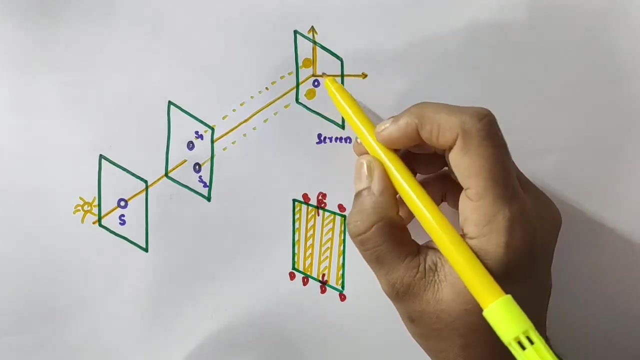 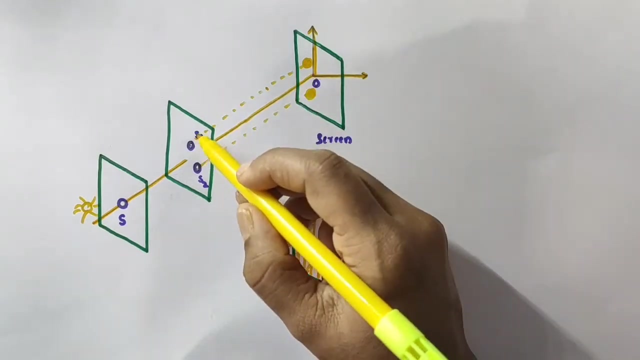 corresponding to S1.. So we expect a bright region corresponding to S1 here on the screen and we expect a bright region corresponding to S2 on the screen. Ok then, in all other regions, that is, this middle region between these two bright regions. again in the middle region, I mean middle region means the middle region of these two. 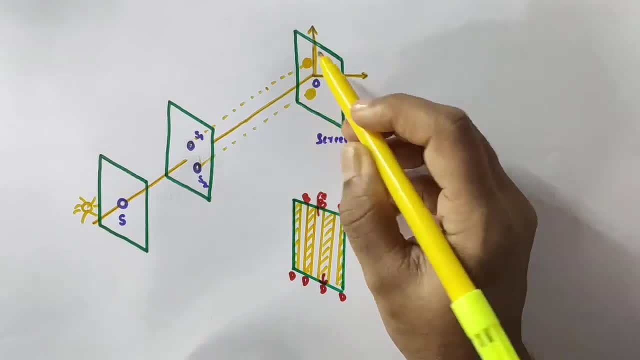 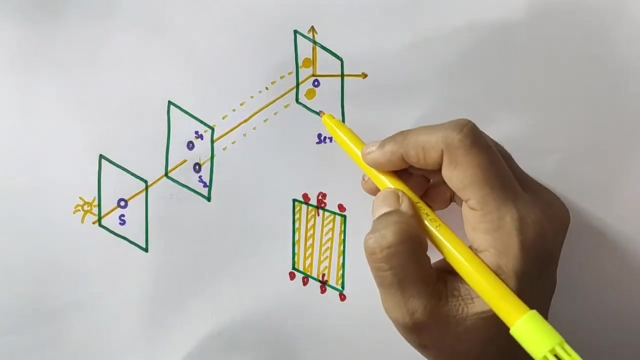 holes S1 and S2.. Ok, in the middle region, in this region, in this region, in this region, in all other regions, we expect a dark, I mean we expect a dark regions here. that is, the shadow of this object or shadow of this opaque object was expected here, That is, at these: 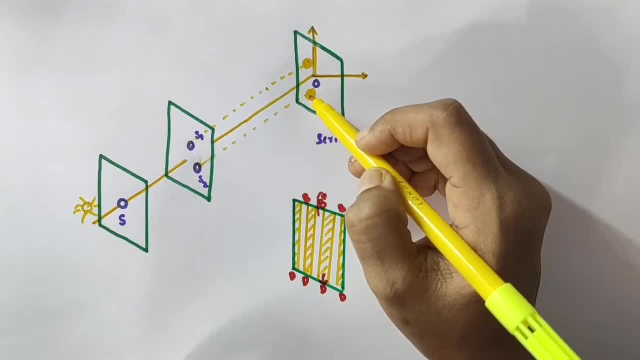 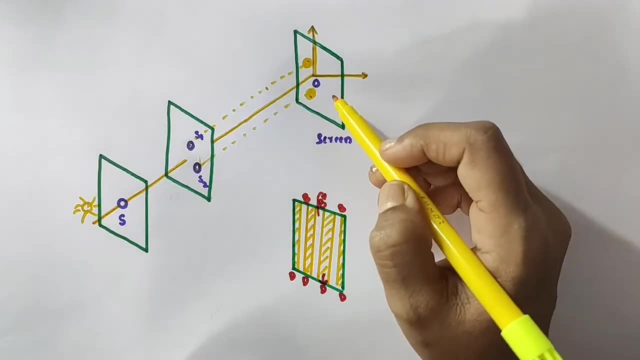 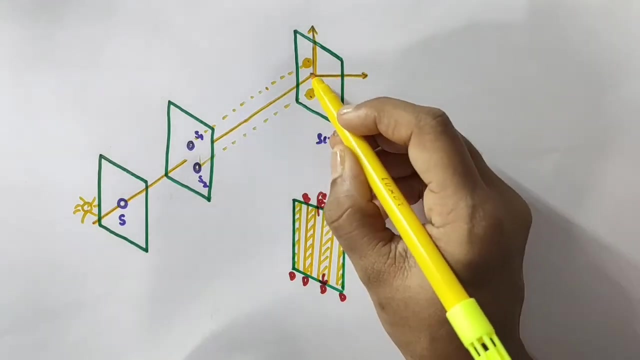 two regions we expect maximum intensities, but this and in all other regions we expect minimum intensities. But this is not what happened there. He, that is, Thomas Young, observed a bright band of light here at the center. He observed a bright band of light here at. 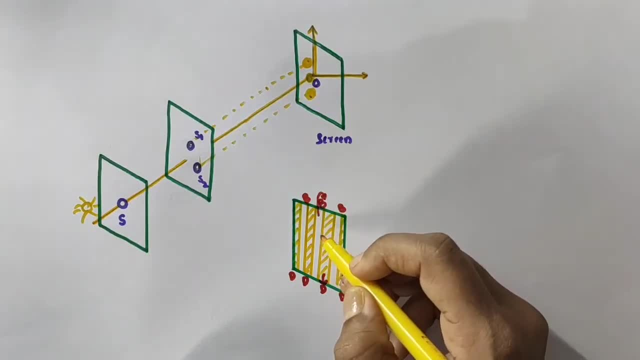 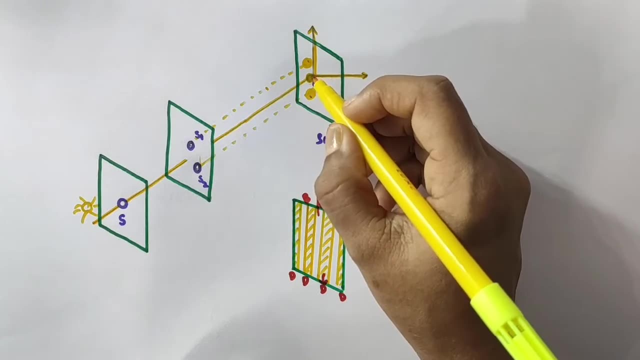 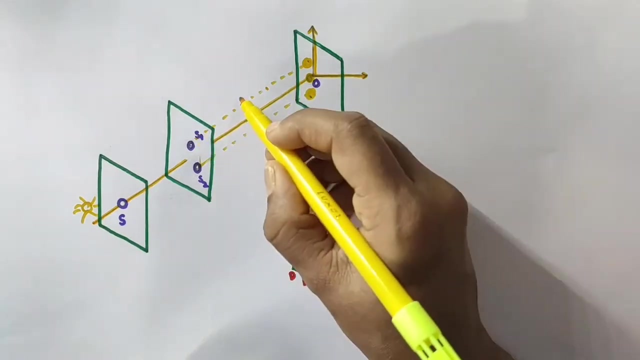 the center. Ok, bright band of light here at the center. And I mean where actually? he observed a bright band of light here at the center where the light rays do not reach when we consider light as rays or particles. You see, when we consider light as a ray, it reaches. 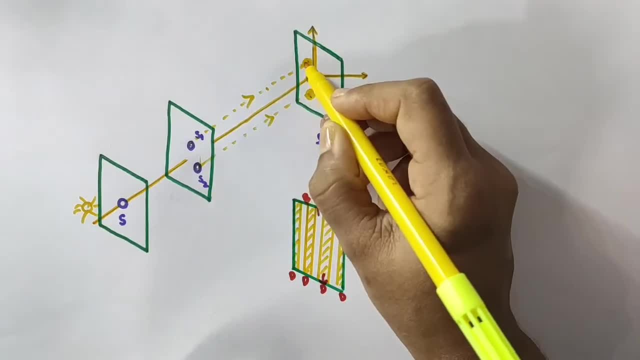 here. When we consider this light as a ray, it reaches here. only These two light rays are not reaching at the center. These two light rays are not reaching at the center. So when we consider light rays- I mean when we consider light as rays or particles- these 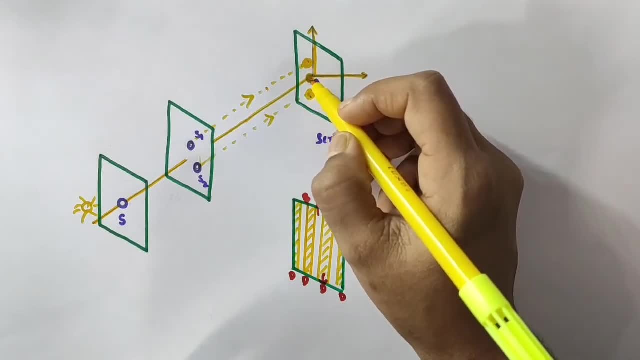 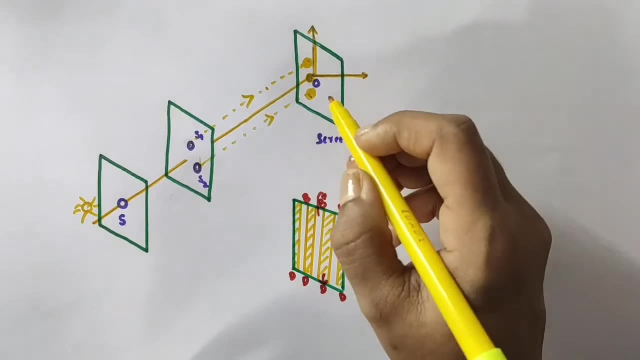 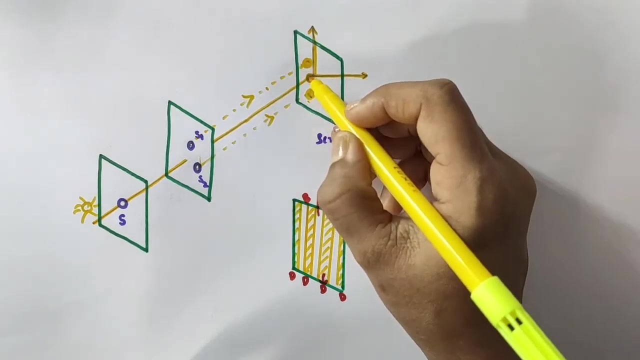 light rays are not reaching at this particular point, at the center point. But Thomas Young observed a bright band of light here at the center. Ok, that is, he observed at the center of these two a bright band of light and alternative bright and dark bands of light on both the 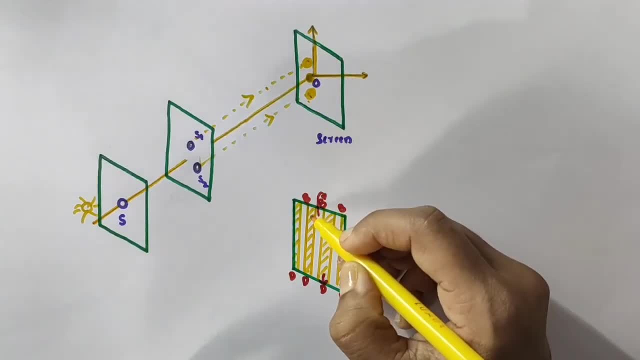 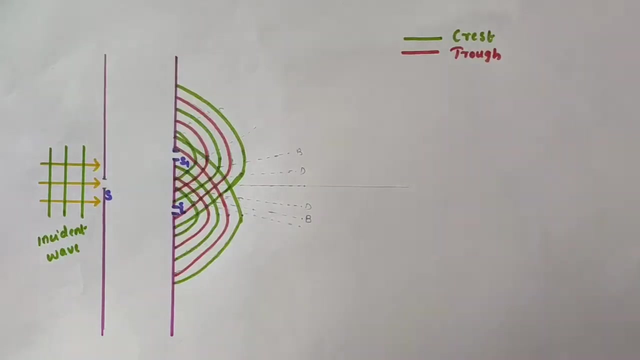 sides. He observed a bright band of light at the center and alternative dark, bright, dark, bright like that. Okay, here also: dark, bright, dark, bright like that. He observed alternative dark, bright and dark bands of light on the both the sides. Actually, this is because of the wave. 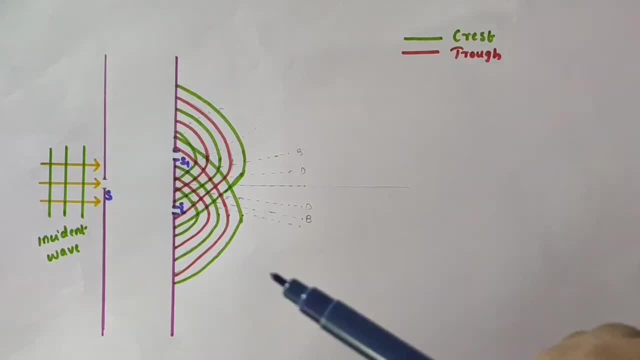 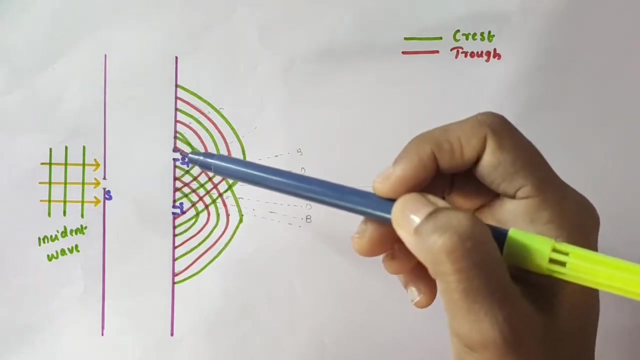 nature of light. Only if we consider light as a wave we can explain this. See, light is considered as a wave here. This is an incident plane wave After passing through these two pinholes. okay, or you can consider two slits here. One is S1, another one is S2.. Either you can consider two. 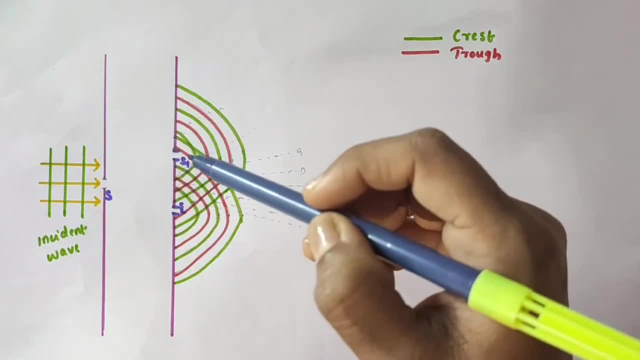 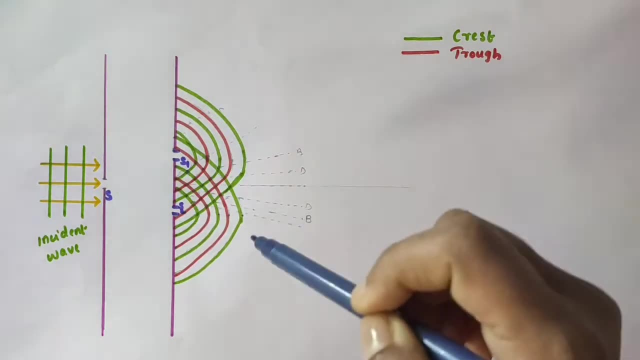 pinholes or slits. and here you see these green lines. no, they represent the crust of the wave and these red lines actually represent the trough of the wave. Alright, and there are waves spreading out from this source S1, and there are waves spreading. 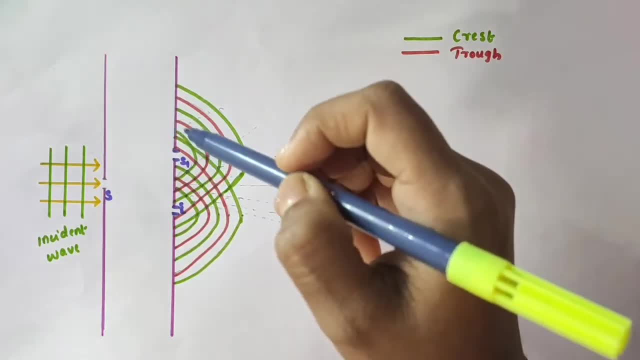 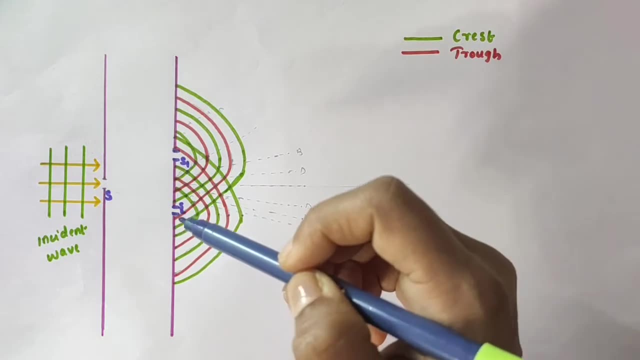 out from this S2 also. Okay, there are waves spreading out from this pinhole S1 or slit S1 as well, as there are waves spreading out from this pinhole or slit S2.. Okay, as we discussed in our previous video, interference of light waves take place here. See, at this particular point, crust. 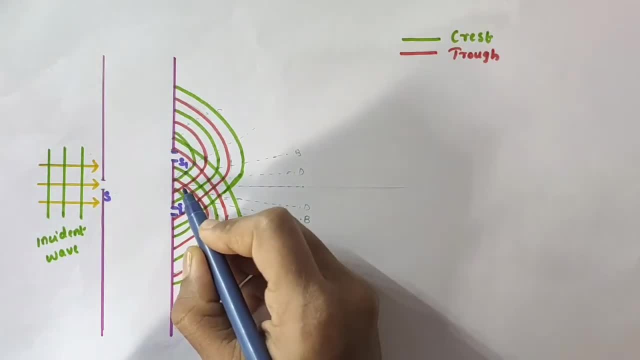 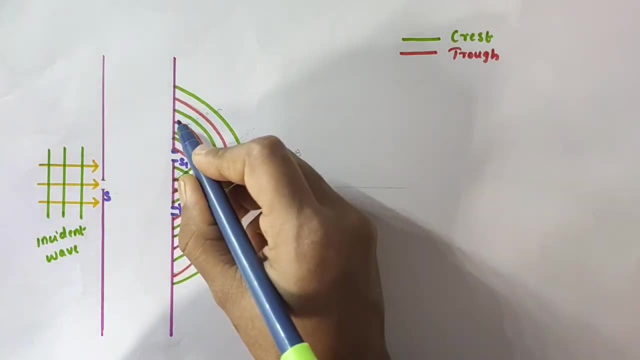 I mean, this is actually trough. no, red one is trough. Okay, so trough of one wave meets the trough of the other. Okay, this wave is actually spreading out from this pinhole S1 and this wave is actually spreading out from the pinhole S2.. So, trough of this wave and trough of this wave, they are meeting here. 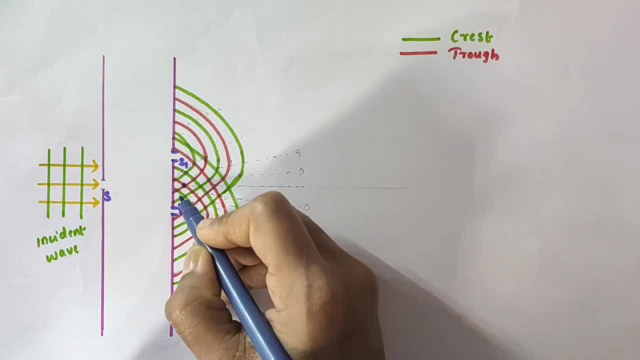 Okay, so constructive interference will take place here. Okay, then, at this particular point. okay, this green one is the crust, So crust of one wave meet the crust of the other wave. This wave is actually spreading out from this pinhole S1 and this. these two pinholes actually act like sources. 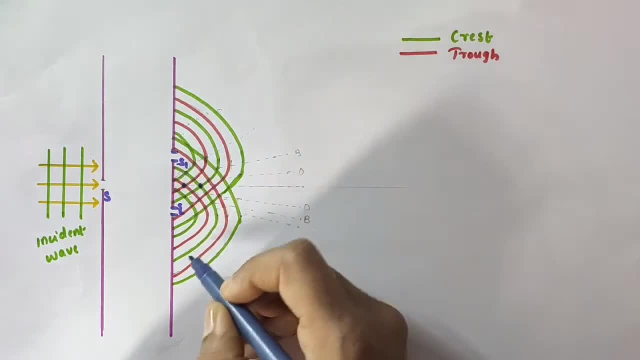 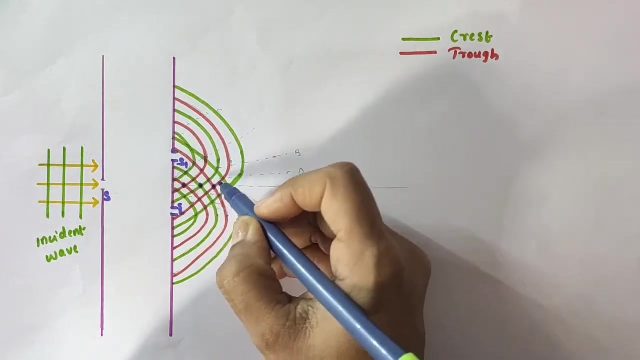 Okay, so this wave actually emanating from this source S1 and this wave is actually emanating from this source S2.. So the crust of this wave meet the crust of this wave. So again, constructive interference will take place here. Okay, next you consider this point Here, the trough of a wave. 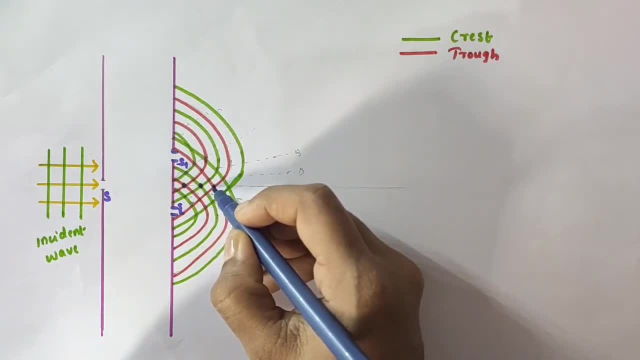 meet the trough of the other. Again, constructive interference take place here And here. you see, you can see that the crust of this wave meet the crust of the other wave emanating from this pinhole S2.. Okay, so, again, constructive interference take place here. So, at all these. 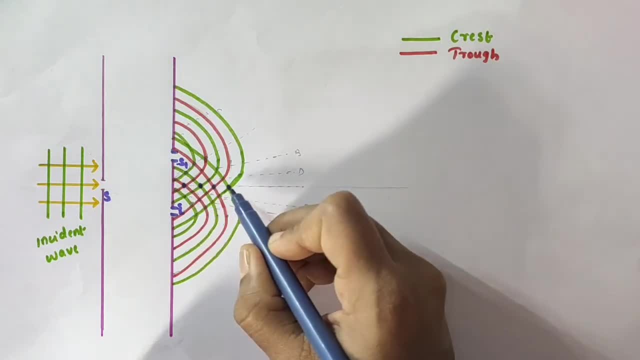 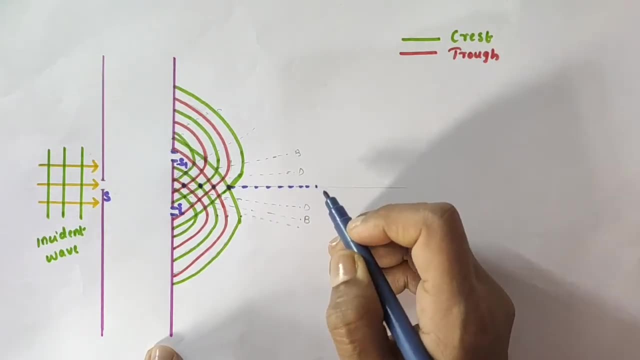 points. constructive interference take place, constructive interference of light take place and, corresponding to this, corresponding to this, we will get maximum intensity of light, because constructive interference of light is taking place here. no, So, corresponding to this, we will get maximum intensity of light. 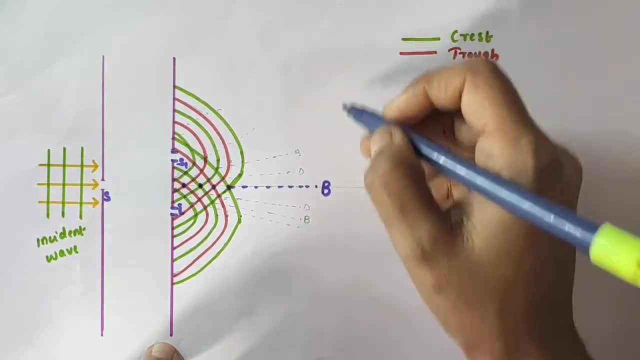 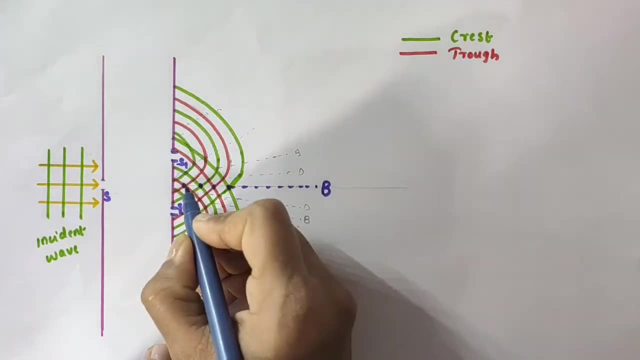 Okay, next see next to this, you can consider this particular point. Here you can see that the trough of the wave emanating from S1 meet this particular point, Okay. trough of the wave emanating from S1 meet which is that point, This point, no, Okay. the crust of the wave emanating from S2.. 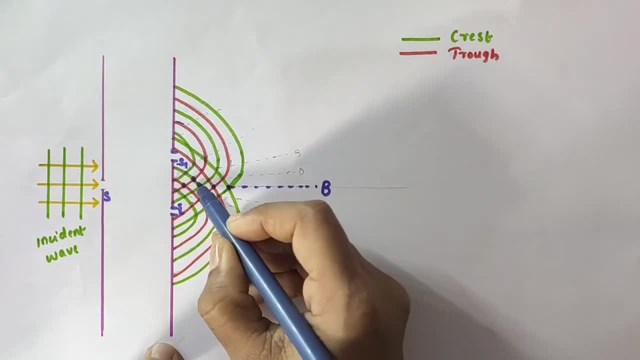 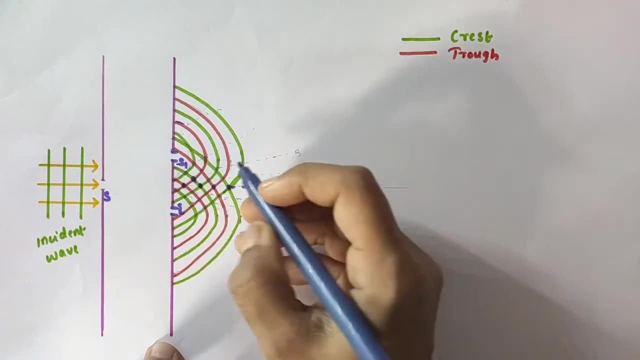 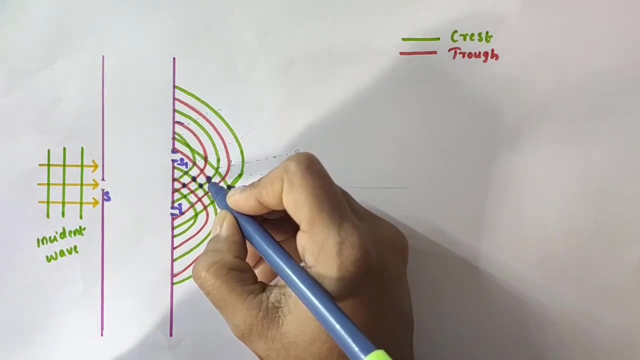 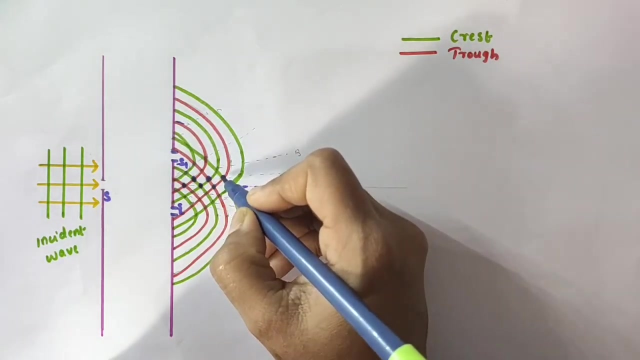 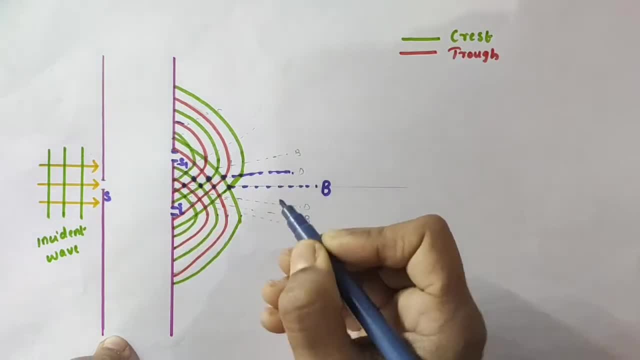 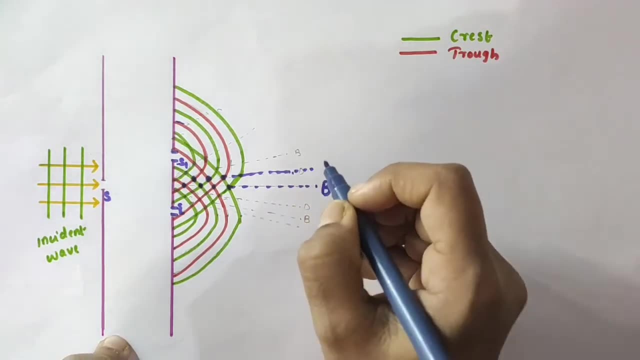 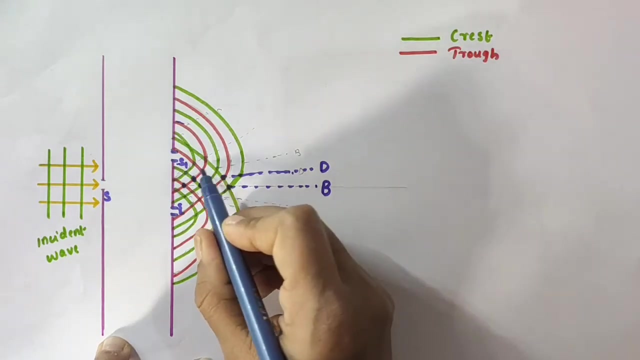 points. at all these points, destructive interference is taking place here. So, corresponding to this, we will get a minimum intensity of light, hence a dark band of light on the screen. Okay, similarly, you can take some other points here. You can see the next to that, you can see. 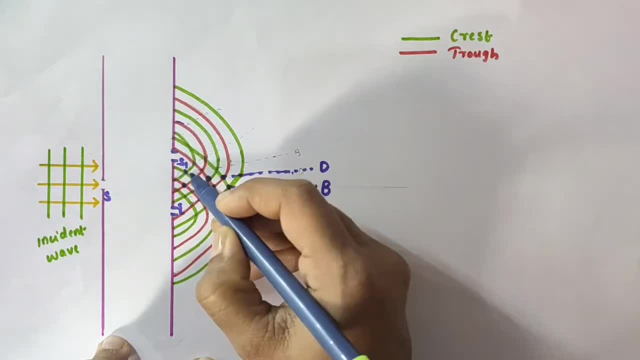 that the crest of this wave and crest of this wave are meeting here. So constructive interference is taking place here. Truff and trough meet here, Crust and crust meet here. So, corresponding to this, we will get a bright band of light because constructive interference are taking place now. 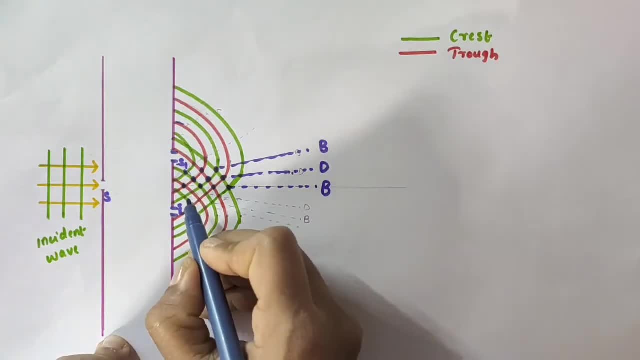 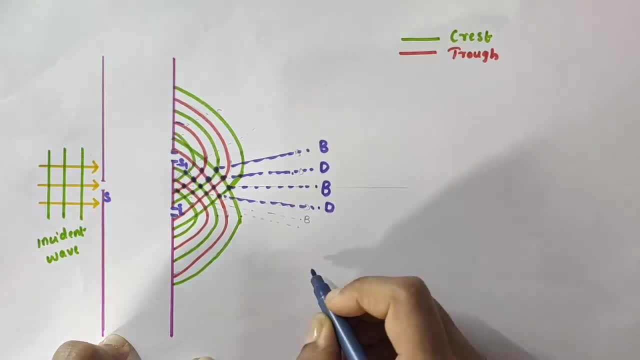 are taking place here. So corresponding to that, you will get a dark band of light. All right, Then next you can consider the next points here, See: crust and crust meet here, Truff and trough meet here, Crust and crust meet here. So corresponding to that you will get, I mean, 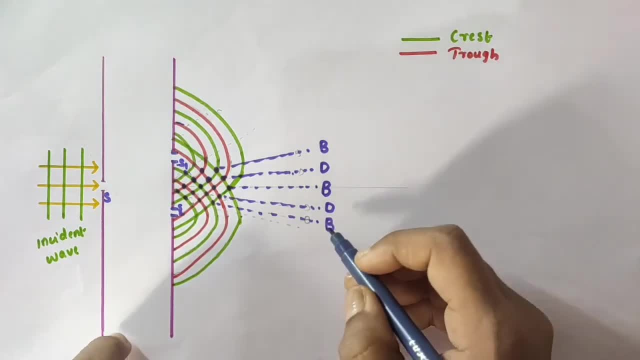 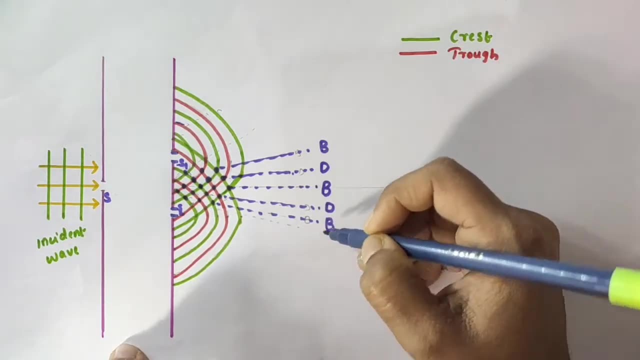 constructive interference is taking place, So you will get a bright band of light. So at the center, on the screen, at the center, you are getting a bright band of light and alternative dark and bright bands on both the sides. Okay, so this theory was a clear proof of wave nature of light. 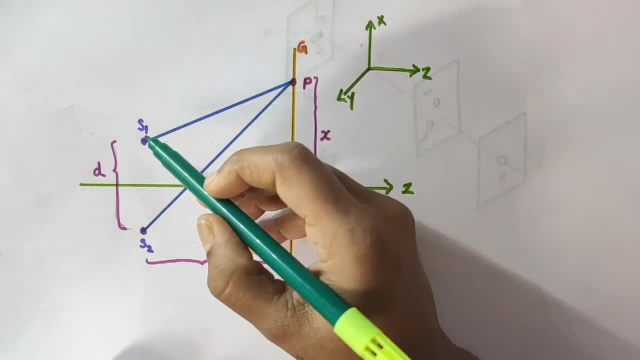 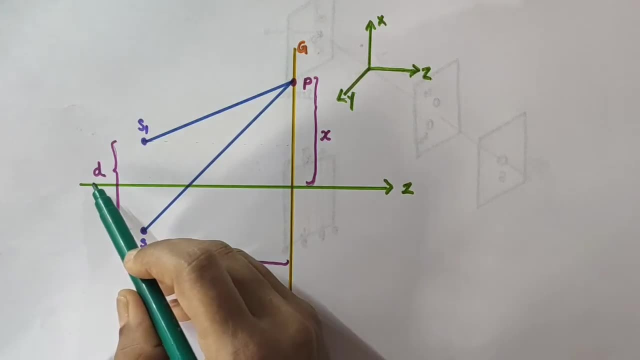 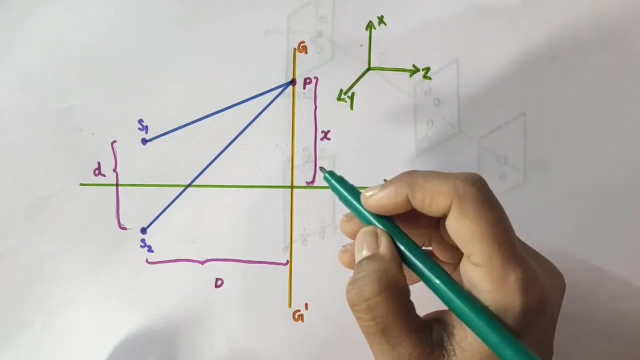 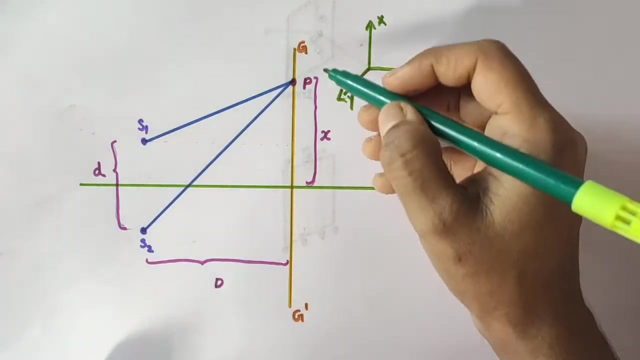 Now see here. these two are two pinholes or two slates, S1 and S2, separated by a distance, small letter D. Here we have a screen GG dash. this yellow one is the screen GG dash, which is D distance, cap letter D, distance away from the two pinholes. Okay, the distance from the pinholes to the screen. 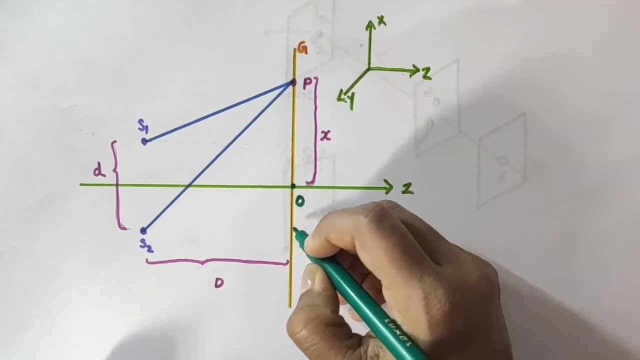 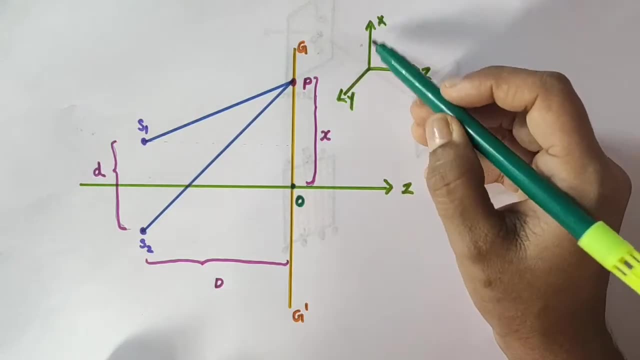 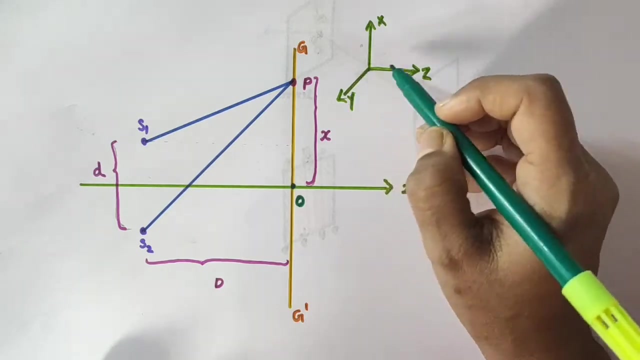 is cap letter D. I am taking this point as O. Okay, See, here we have taken this line as along the- I mean X axis. Okay, here this is the coordinate system considered here. This one is along the X axis. This one is taken as X direction, Y direction. 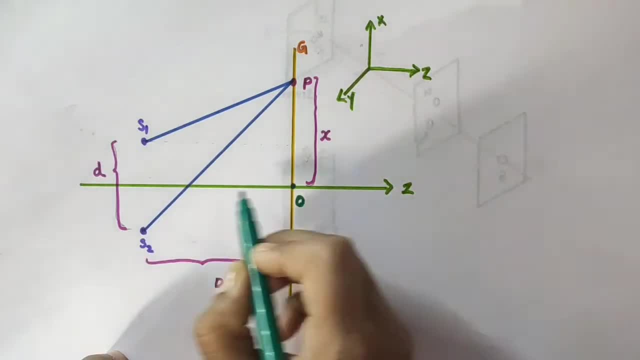 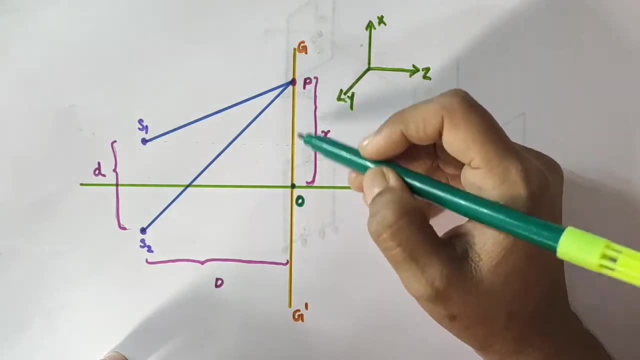 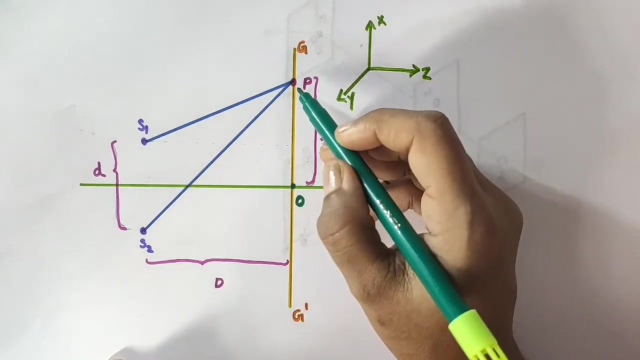 and the Z direction. So here see this line, this horizontal line O. This line is taken as along the Z axis and this as along the X axis. Okay, and the distance from this point O to any arbitrary point P on the screen, GG dash, that is taken as small letter X. 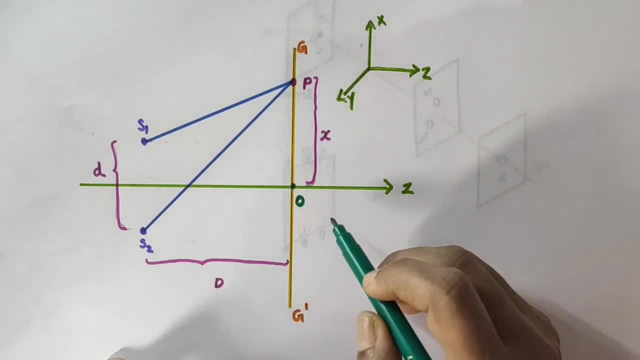 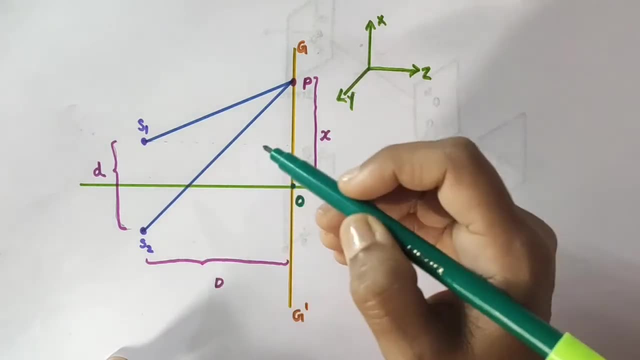 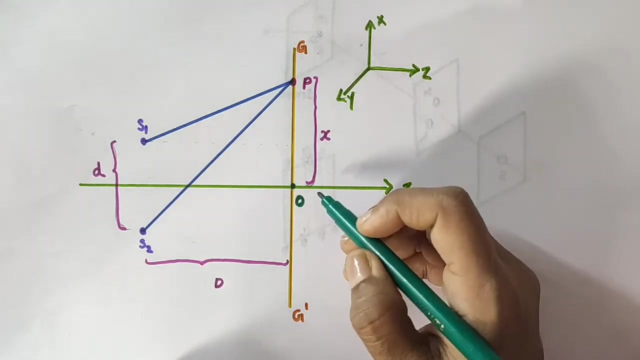 So from the concepts we discussed so far in this video, we know that the spherical waves emanating from S1 and S2 will produce interference fringes on the screen. GG dash. Now, how can we determine the positions of maximum and minimum intensities? where would 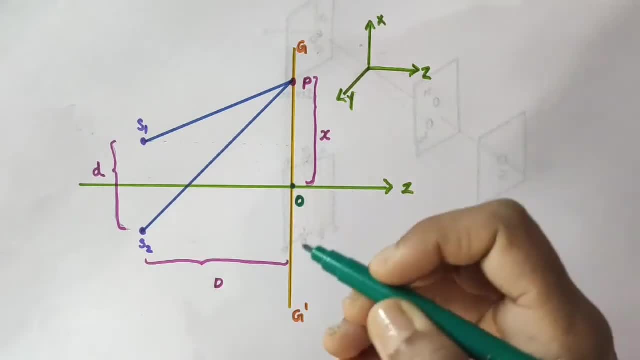 be getting a bright band of light or what would be getting a dark band of light? How can we determine that position of maximum and minimum intensities of light? for that, Consider an arbitrary point P on the screen, that is, on this line: GG dash. 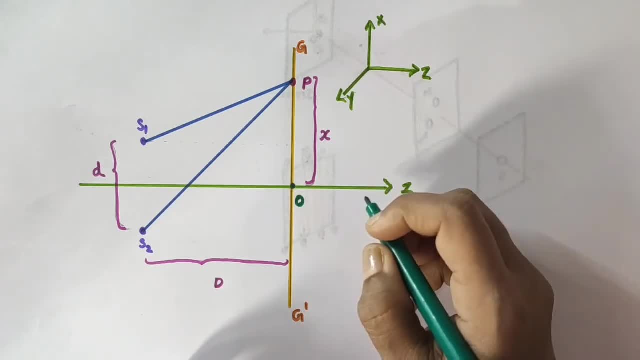 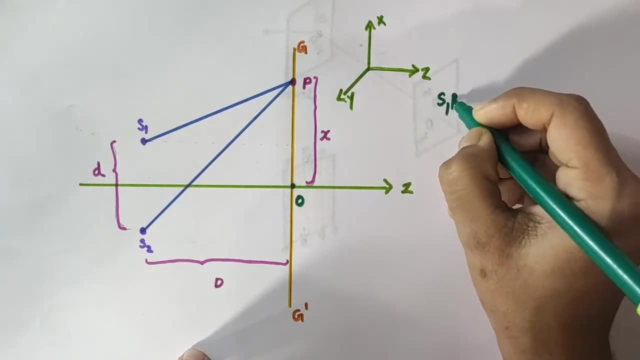 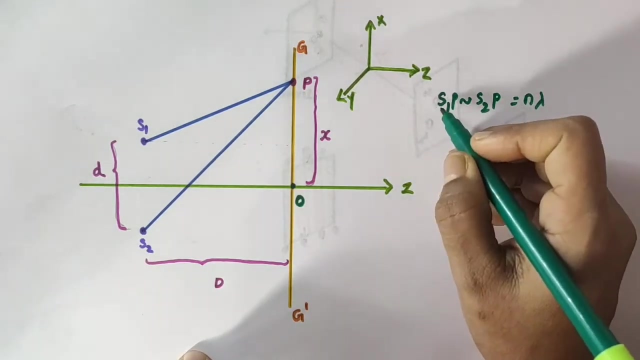 In our previous video we have seen that at any arbitrary point P, the condition for the constructive interference is S1P- S2P 0. That is, you can consider S1P minus S2P or S2P minus S1P. 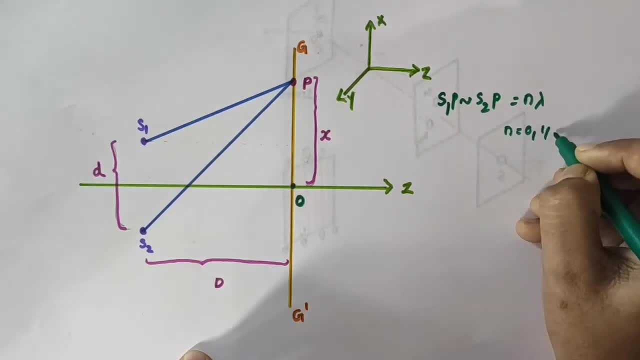 That is what the sign indicate, where N equal to 0,, 1,, 2,, 3, etc. 1,, 2,, 3, etc. Okay, I will provide the link for this in the description box. If you want, you can watch that. 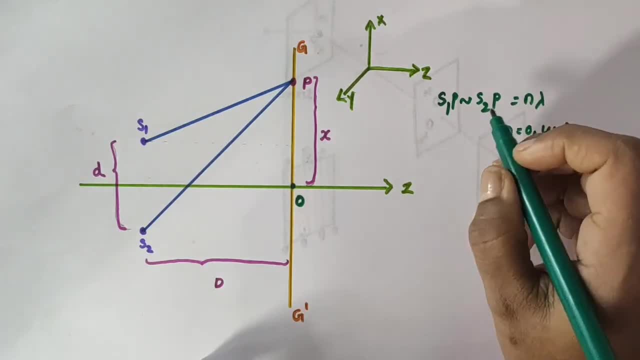 We have discussed this in our previous video. Okay, so at any arbitrary point P on the screen, the condition for the constructive interference is S1P. S2P is equal to N lambda. This sign actually indicates that you can either take S1P minus. 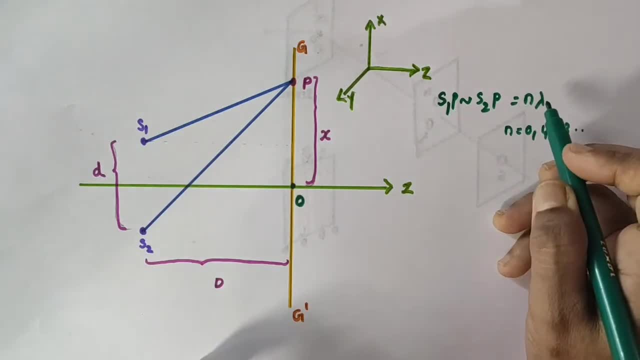 S2P or S2P minus S1P, that must be equal to N lambda. for constructive interference to take place where N equal to 0,, 1,, 2,, 3, etc. That is for constructive interference. the path difference needs to be N lambda. 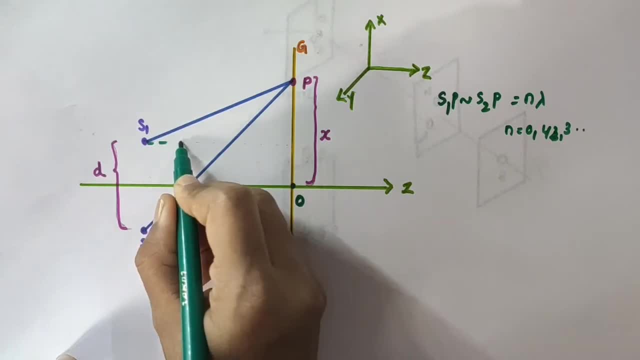 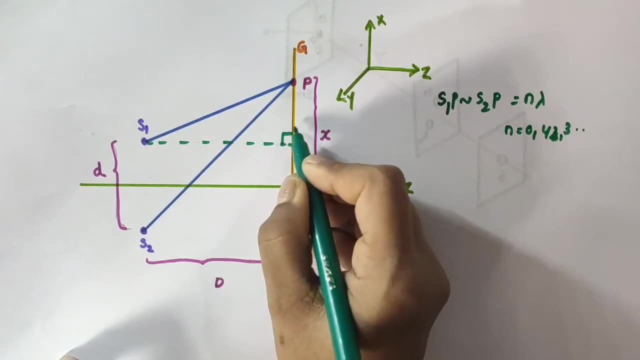 Okay, now see, here I am just forming a triangle. Okay, I am just forming a triangle. What about this angle? This angle is 90,. no, So here we have a right angled triangle. Okay, I am considering this triangle. 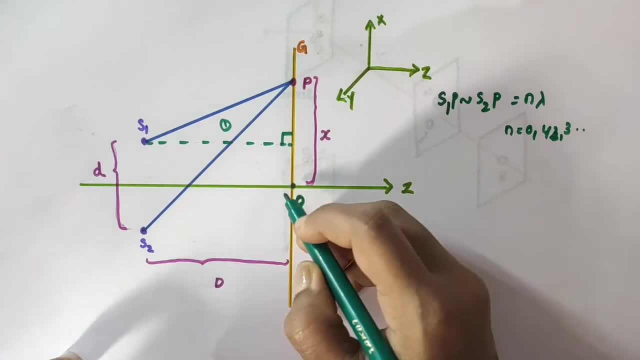 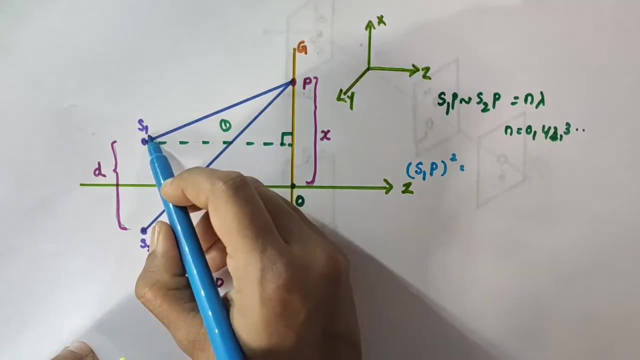 I am taking it as triangle 1.. Okay, this one Right angled triangle. Then in this triangle, what about S1P? square S1P means this one That is a hypotenuse of this is 90.. So opposite side is hypotenuse. 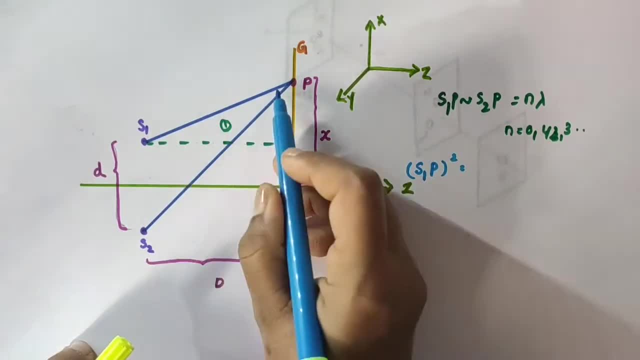 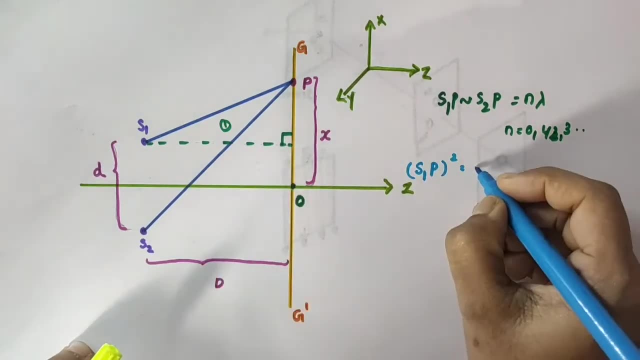 So S1P is a hypotenuse of this right angled triangle. So in this triangle S1P square is equal to base square plus altitude square. So this side is of length capilator D, So D square plus what about this? 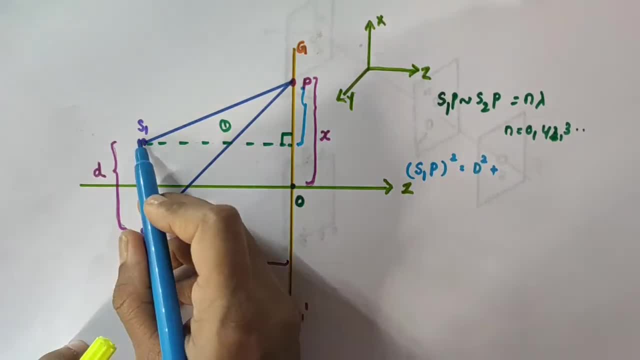 This length. See, this is I mean S1 and S2 are separated by a distance, D. So what about the distance from here to here and from here to here? This is D by 2 and this is also D by 2.. 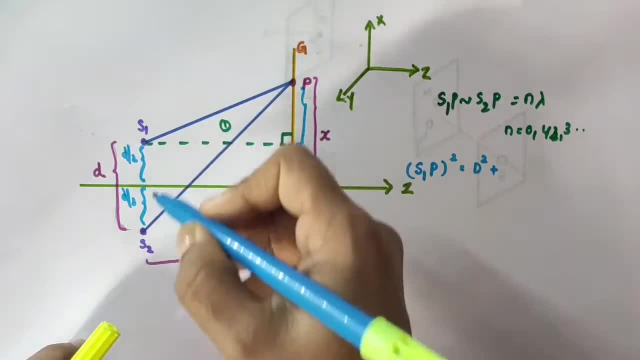 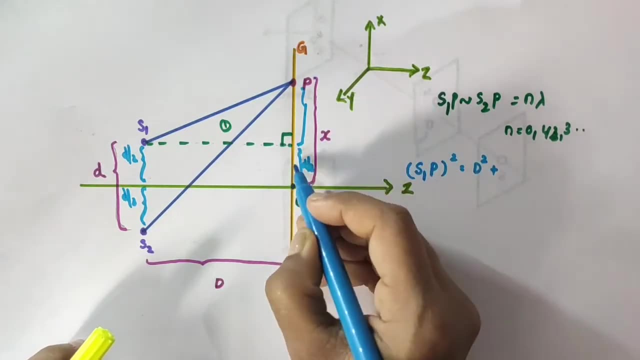 Okay, they are arranged in that manner. Okay, S1 and S2 are kept in that manner. Alright, so this distance is D by 2.. Okay, from here to here X, this distance is D by 2.. I hope you can see the D by 2.. 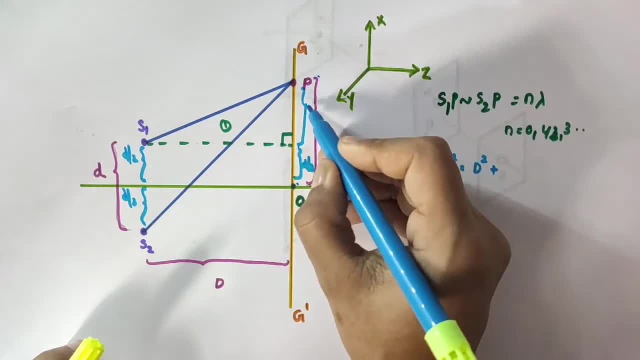 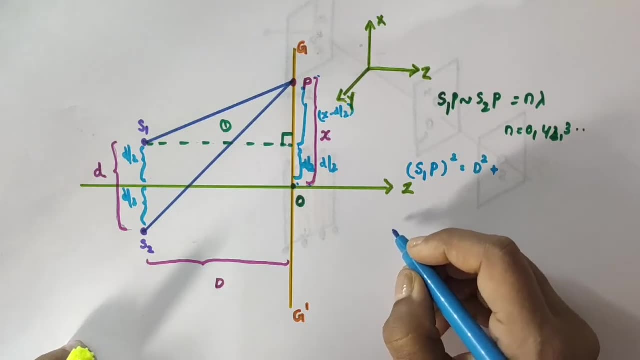 Okay, from here to here D by 2.. From here to here X. So what about this distance? That would be X minus D by 2.. This distance would be X minus D by 2.. Okay, so here we can write X minus D by 2, the whole square. 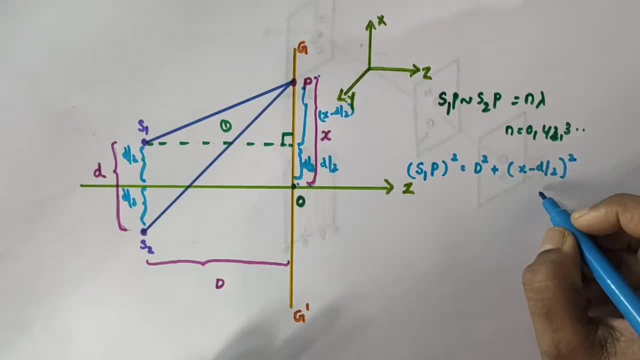 Okay, from Pythagoras theorem, we are getting this. I am taking this as see, I am taking this as equation number 1 and I am taking this as equation number 2.. Alright, next I am forming an another right angled triangle here. 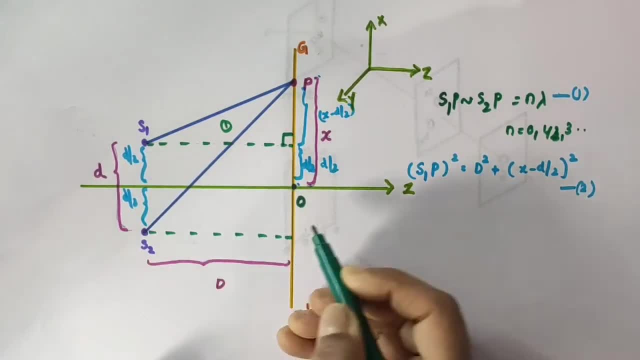 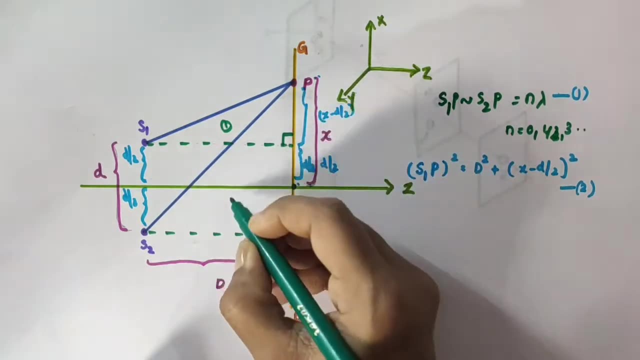 See, I am forming a right angled triangle here. That is this one, Okay, this big one. What about this angle? This angle is 90. So this is a right angled triangle. I am just naming it as 2.. 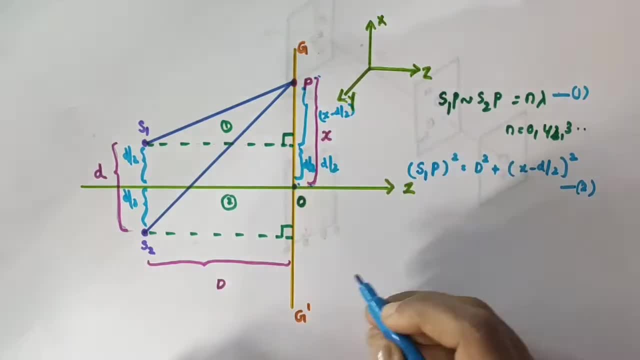 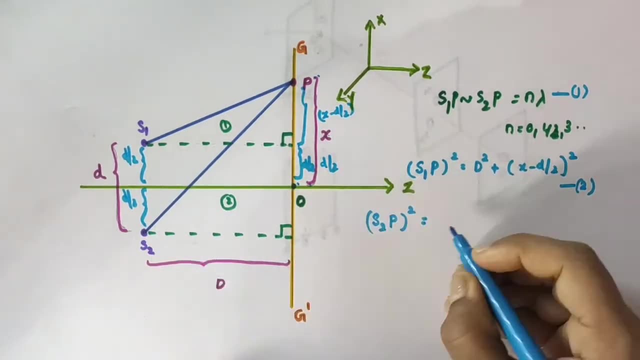 Okay, so here the hypotenuse is what S2P? So here when we apply the Pythagoras theorem, we can write: S2P, square is equal to this side, That is D, D square plus from here to here. 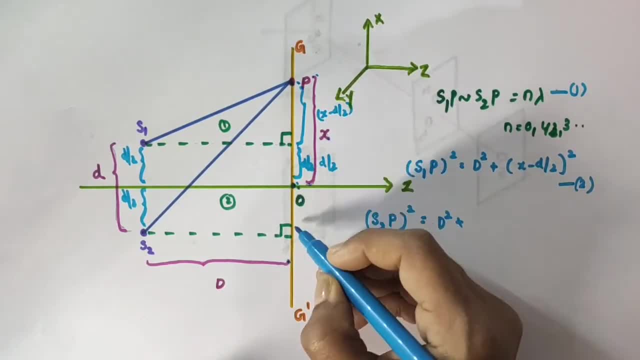 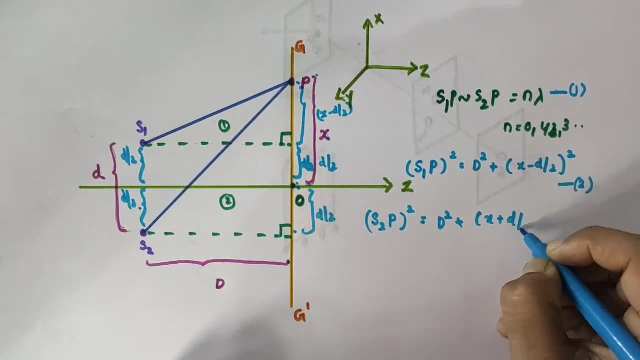 What about? from here to here? That is X. Then from here to here, D by 2.. Okay, this is D by 2.. So X plus D by 2.. X plus D by 2, the whole square. I am taking this as equation number 3.. 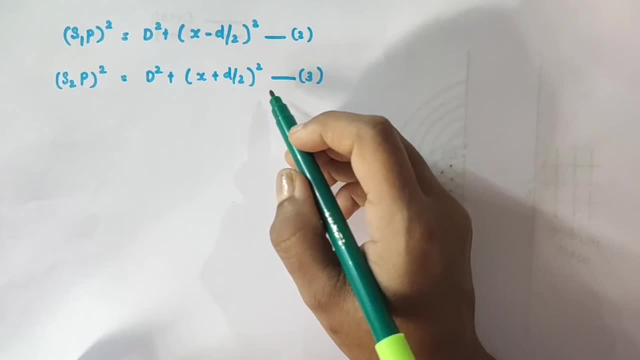 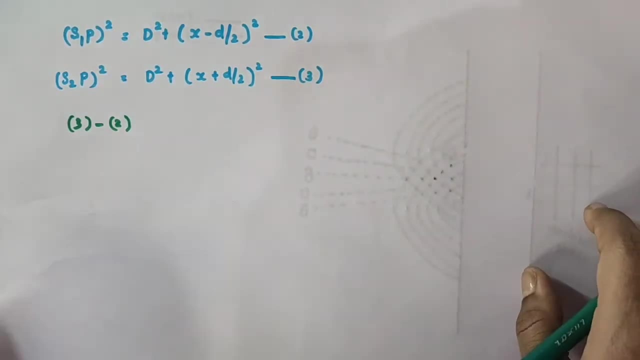 So see, we got equation number 2 like this and equation number 3 like this. Next, what I am doing is I am just subtracting this equation number 2 from equation number 3.. That is equation number 3 minus equation number 2.. 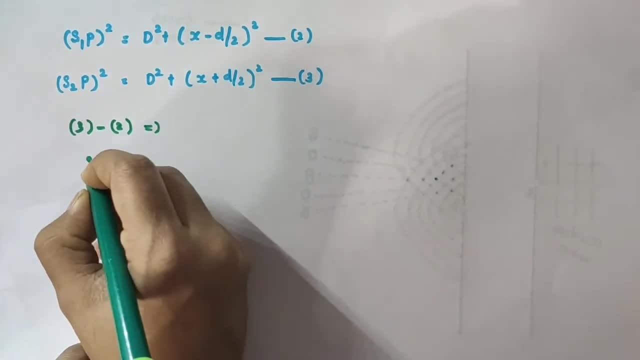 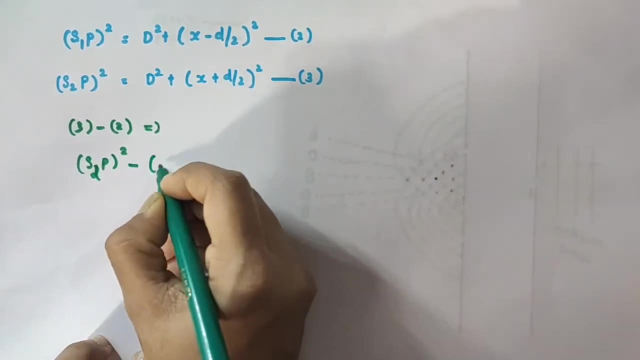 Alright, so this implies S1P square, S1P square. Okay, equation number 3 minus 2 now, So S2P, S2P square minus S1P square is equal to what? S2P square is what? 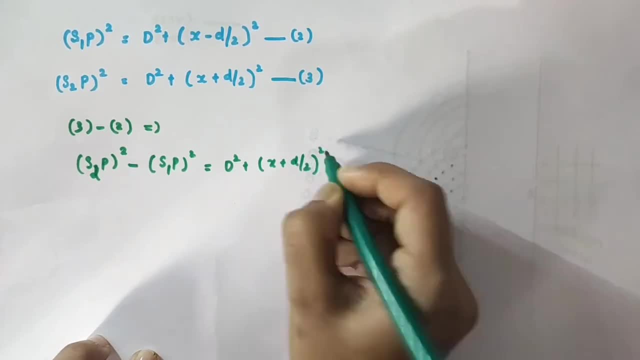 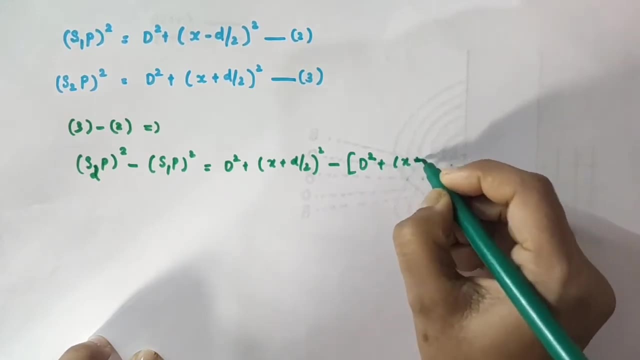 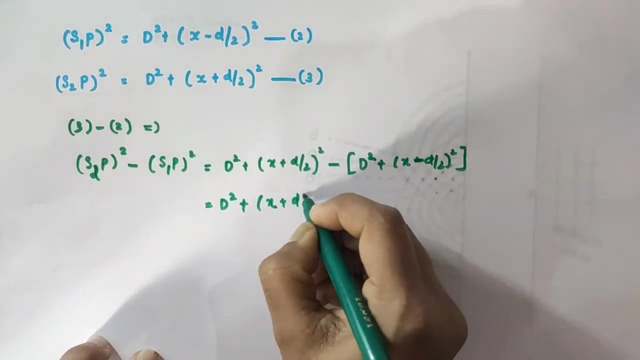 D square plus X plus D by 2, the whole square minus minus of D square plus X minus D by 2, the whole square. Okay, this can be written as D square plus X plus D by 2, the whole square minus D square minus into plus minus. 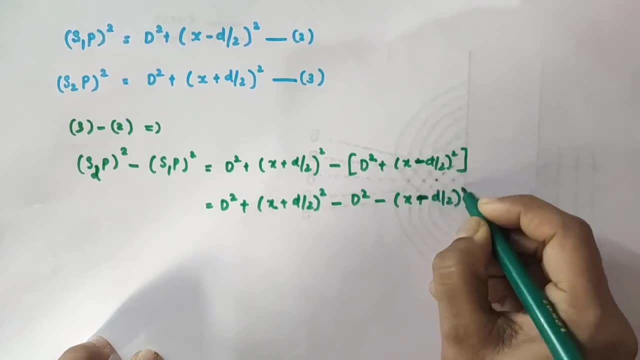 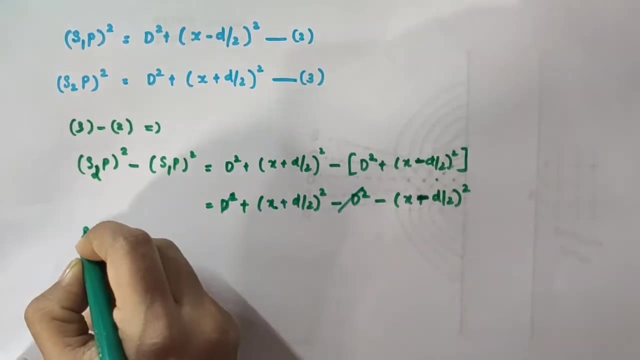 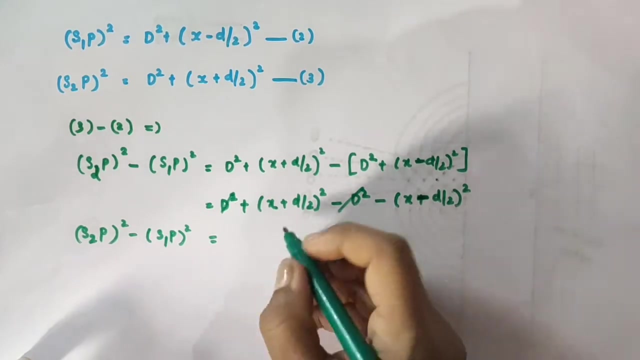 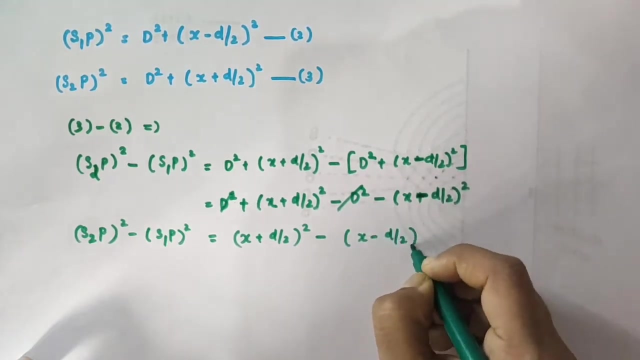 So minus X, plus- I mean sorry X minus D by 2 the whole square. This is minus. Okay, now you see, plus D square, minus D square, cancel. So let us. we have S2P square. minus S1P square is equal to X plus D by 2 the whole square. minus X minus D by 2: the whole square. 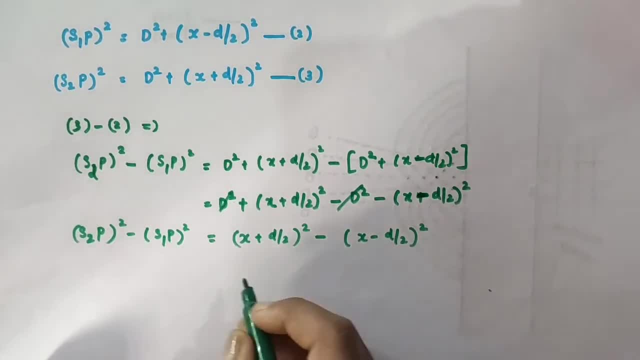 Next, I am just expanding this. Okay, so this becomes A plus B the whole square. Now, A square plus 2AB. okay, plus B square, that is, D by 2 the whole square. Alright, then, minus A, minus B the whole square. 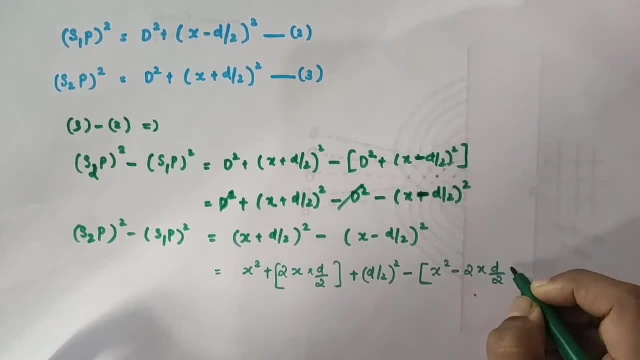 A square minus 2AB. okay, plus B square. So D by 2 the whole square. Yeah, alright, So this becomes X square. Alright, so this becomes D by 2 the whole square. 2, 2 cancel. 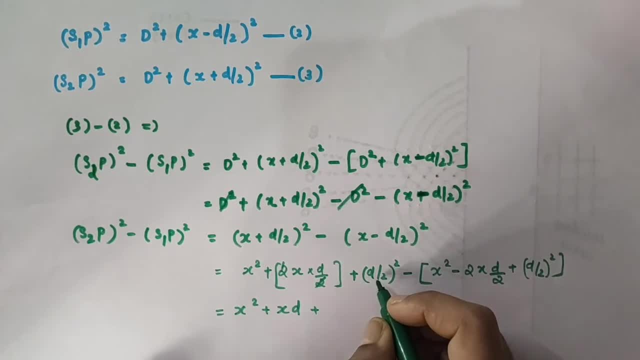 So plus X into D, plus D by 2, the whole square. that becomes what D square divided by 4.. Okay, D square divided by 2 square is 4.. Minus X square, minus into minus plus 2, 2 cancel. 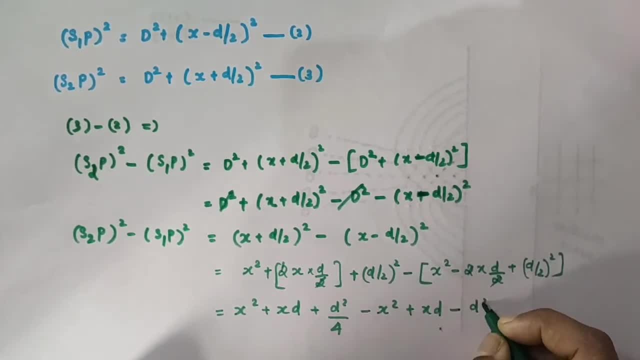 So plus X into D minus, into plus, minus D square divided by 4.. Okay, now you see, plus X square, minus X square can be cancel. Alright, then plus D square by 4, minus X square, Minus D square by 4, minus D square by 4 can be cancel. 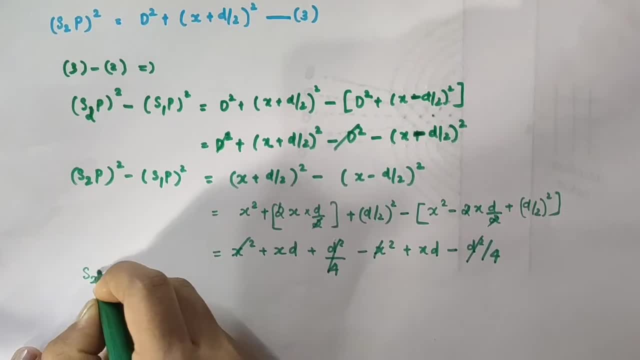 So this equation becomes: S2P square minus S1P square is equal to XD plus XD, that is 2XD. Okay, I am taking this as equation number 4.. Now this is like A square minus B square. no, What is A square minus B square? 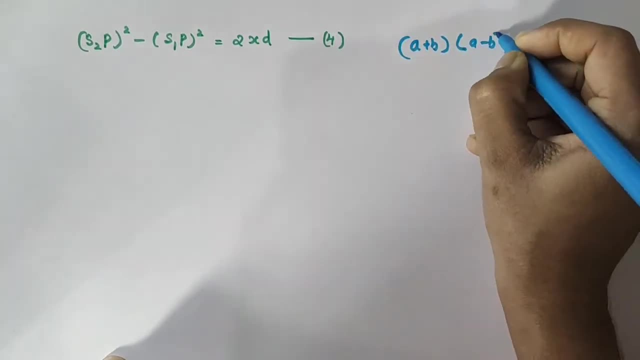 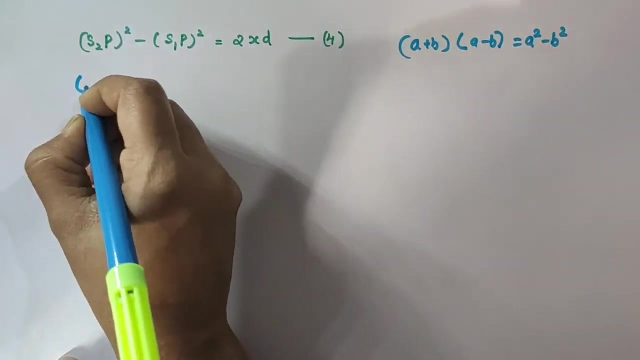 A square A plus B. A plus B into A minus B can be written as S square minus B square. no, So here S2P square minus S1P square can be written as S2P plus S1P into S2P minus S1P. 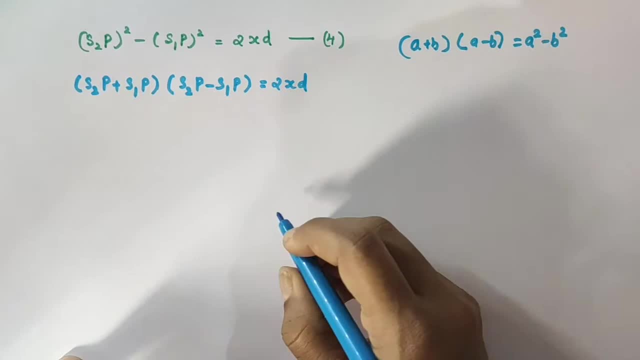 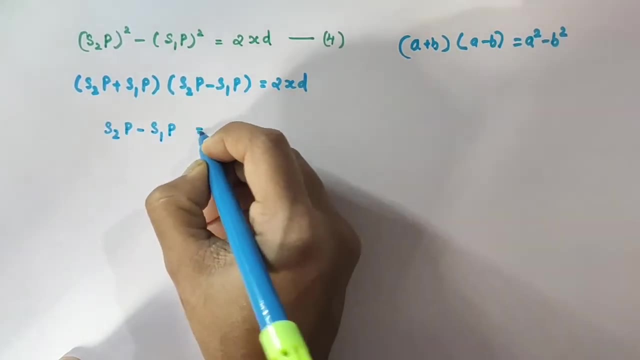 This is equal to what? This is equal to 2XD. Okay, now from this we can write: S2P minus S1P is equal to 2 into X, into D. Divide it by. I am taking this S2P plus S1P to this side. 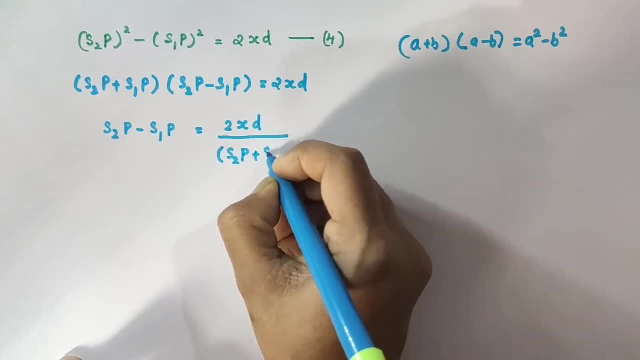 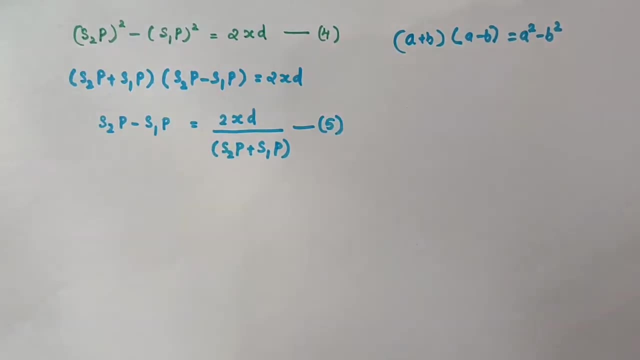 So that goes to the denominator, So S2P plus S1P. Okay, I am taking this as equation number 5.. Now if small letter X, comma D, small letter X was the distance from the point O to the arbitrary point P? 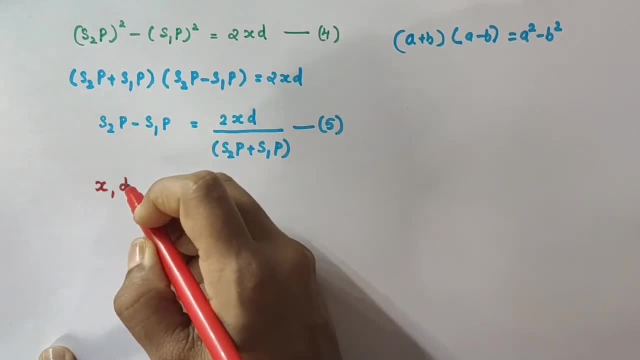 I hope you remember this. And small letter D was the distance or separation between the two pin holes or two slits, S1 and S2.. So if X comma D is very much less than the capital letter D, Capital letter D was the distance between the pin holes or the slits S1 and S2.. 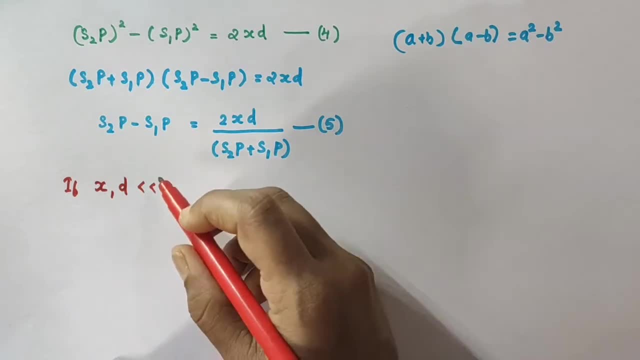 I mean, and the screen? Okay, the distance from the screen to the two S1 and S2, two slits, or the pin holes, that was capital letter D. So if X comma, D is less than both, X and D are less than capital letter D. 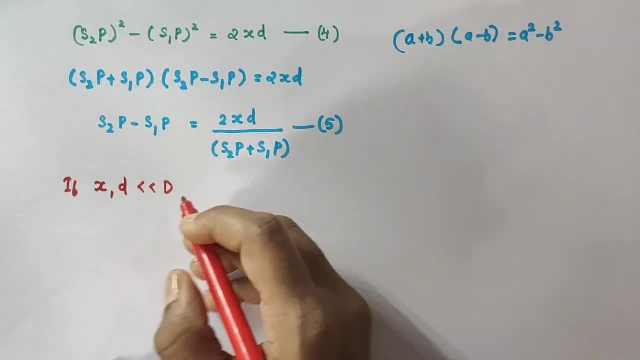 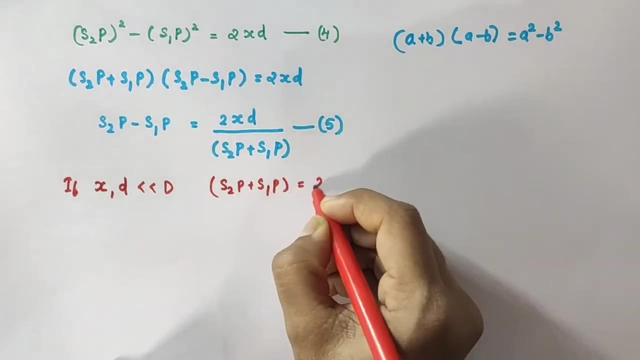 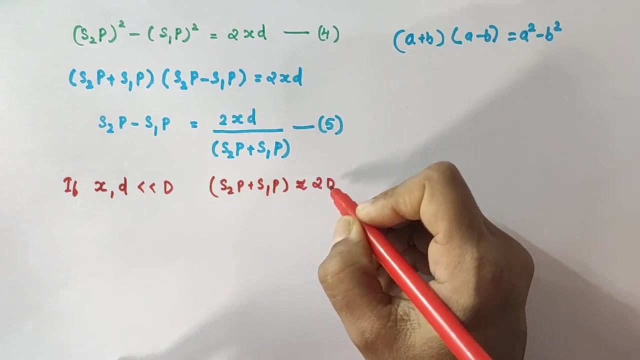 Then negligible error will be introduced. if the denominator of this expression, That is, S2P, S2P plus S1P, is replaced by capital letter, Approximately we are replacing this by 2 into capital letter D. So if you are replacing this denominator by 2D, capital letter D, 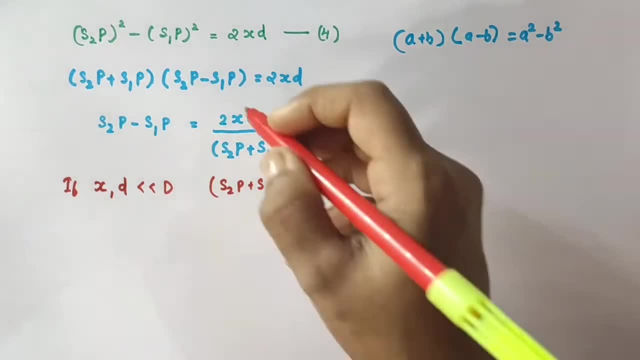 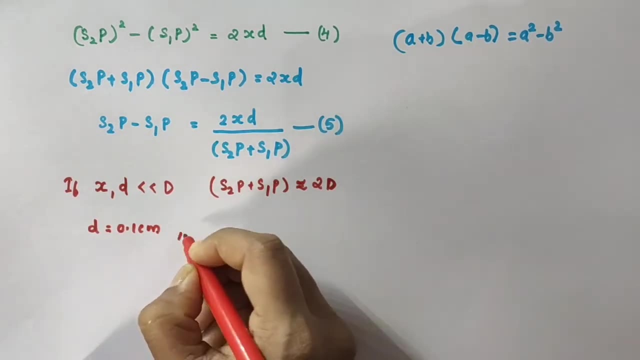 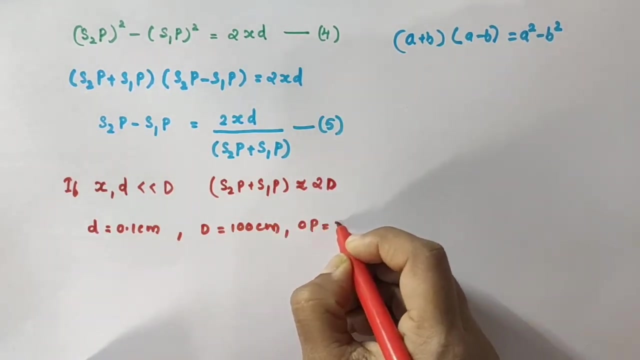 Okay, 2D. Only negligible error will be introduced in the calculation. For example, let small letter D is equal to 0.1 centimeter and capital letter D is equal to 100 centimeter. Okay, then let OP. OP is actually the distance. 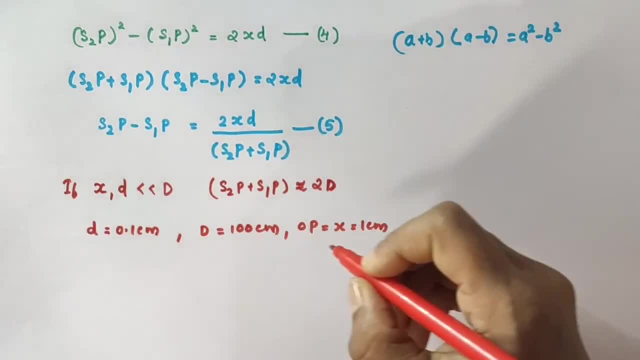 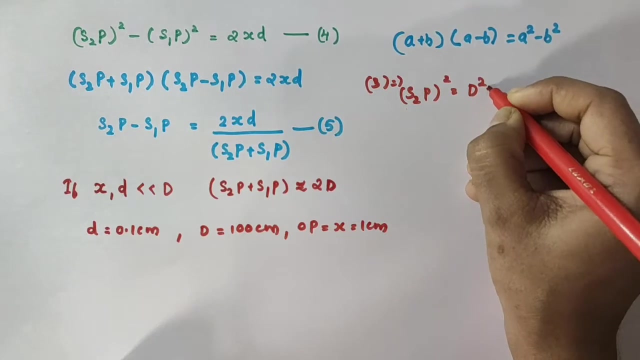 X, which is equal to 1 centimeter. These are actually the typical values for an interference experiment. Alright, now from equation number 3.. I hope you remember that equation number 3.. Equation number 3 was: S2P square is equal to D square plus X plus D by 2, the whole square. 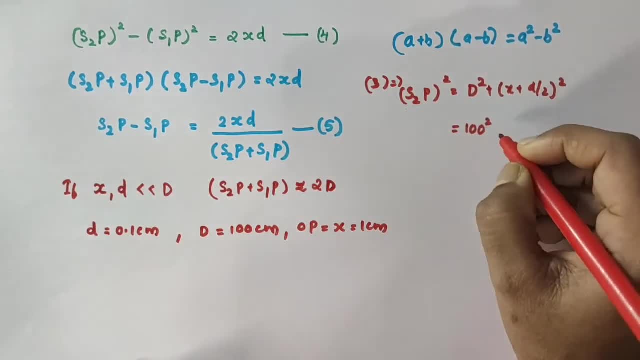 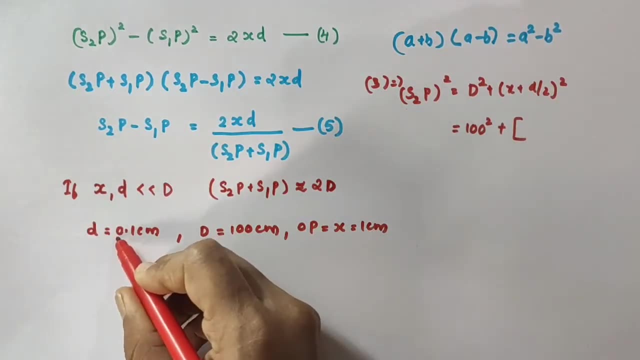 Okay, so here that becomes capital letter. D is 100 centimeter, So 100 square plus X plus D by 2.. X is 1 centimeter, D by 2. D by 2 will be 0 point. This divided by 2 means 0.05.. 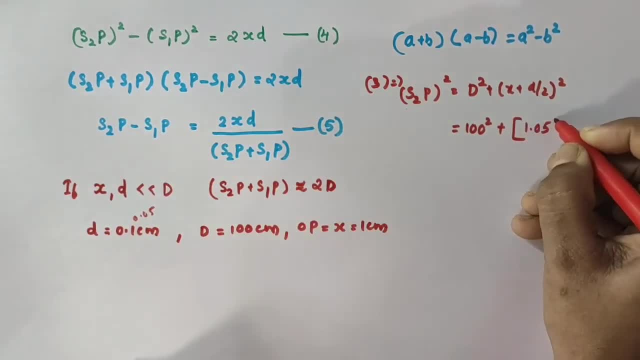 So 1 plus 0.05 is 1.05, all square. All are in centimeters, So I am not taking any unit conversions here, Because all the terms are given in centimeters. Okay so, 100 square plus 1.05 square. 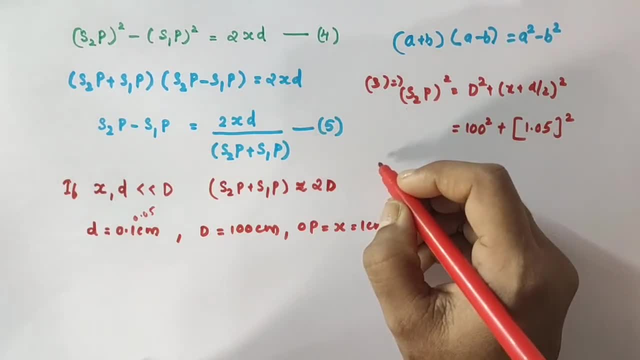 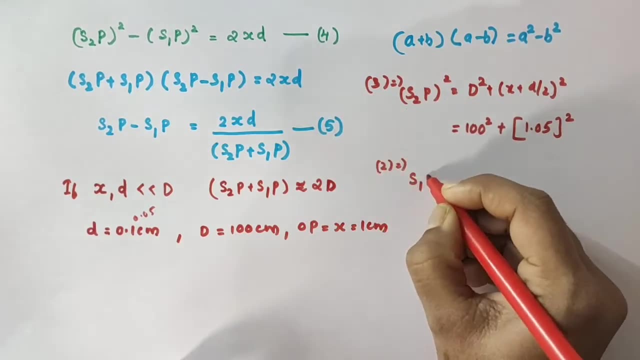 Let it be like this, Next from equation: Okay, then from the equation, I mean from equation number 2. We have S1P square. S1P square is equal to D square, plus X, minus D by 2, the whole square. 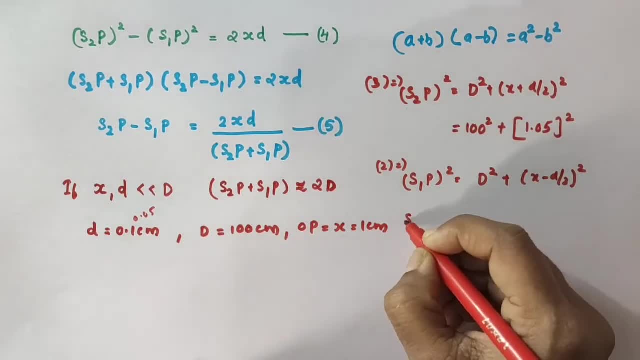 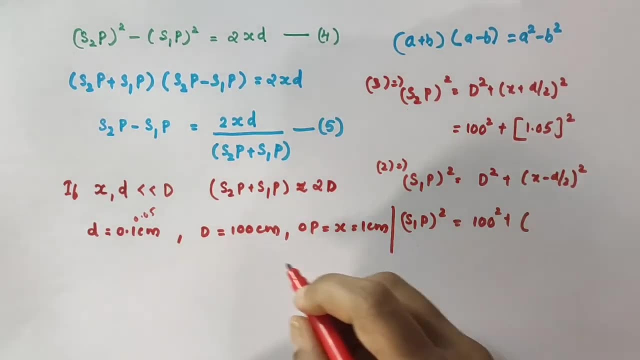 Okay, then when we substitute these values here, This becomes: S1P square is equal to D square, That is 100 square plus X minus D by 2.. X minus D by 2.. 1 minus 0.05.. Okay, that becomes 0.95 square. 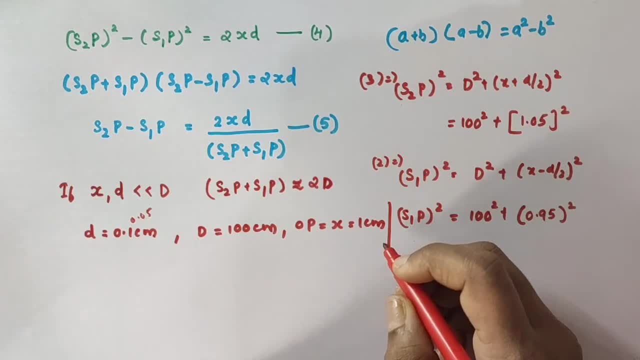 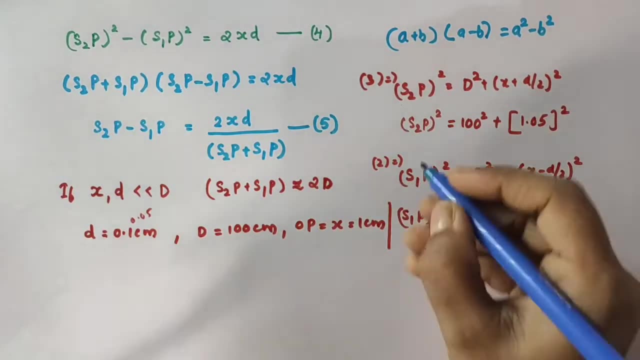 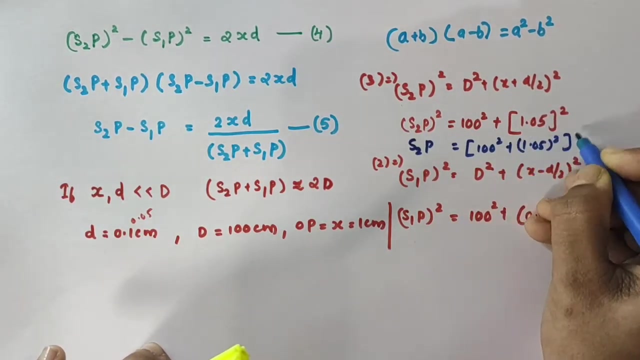 Alright now. Okay, then, from this See, this is S2.. S2P square is equal to this value. So what about S2P? S2P will be 100 square plus 1.05 square, all raised to 1 by 2.. 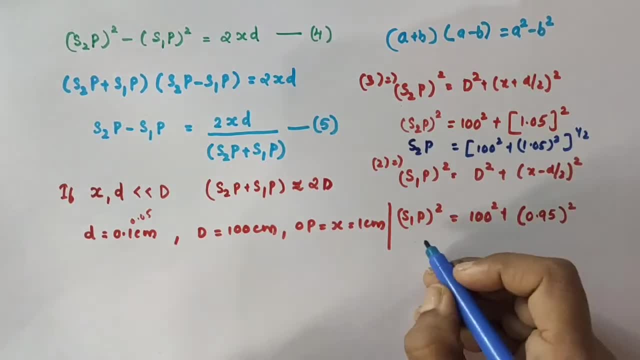 Okay, square root of. Similarly, this S1P square is equal to this one, So S1P is equal to square root of this. That is, 100 square plus 0.95 square, all raised to 1 by 2.. 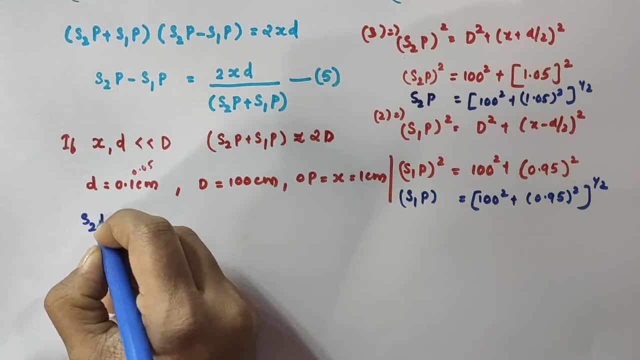 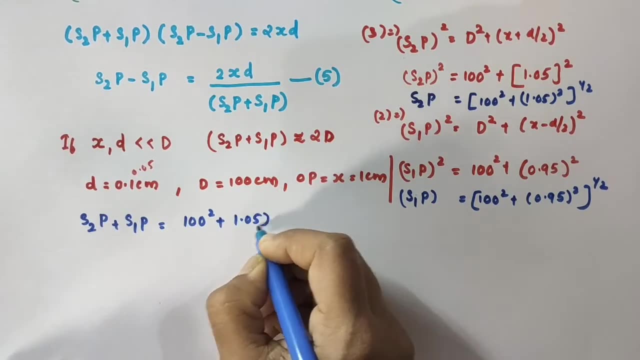 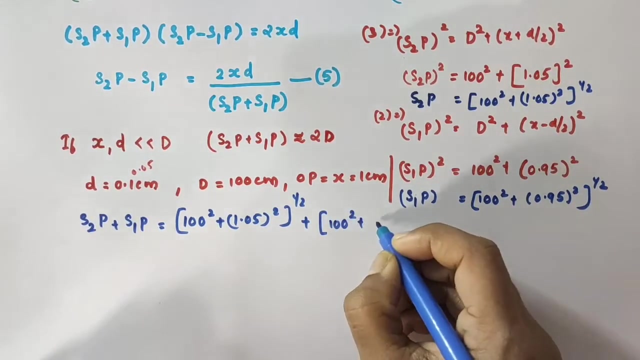 So what about the denominator S2P plus S1P, S2P? we are getting it as 100 square plus 1.05 square, all raised to 1 by 2.. Plus, what about S1P? 100 square plus 0.95 square, all raised to 1 by 2.. 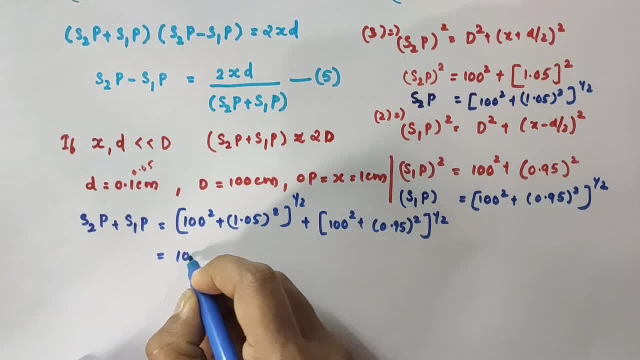 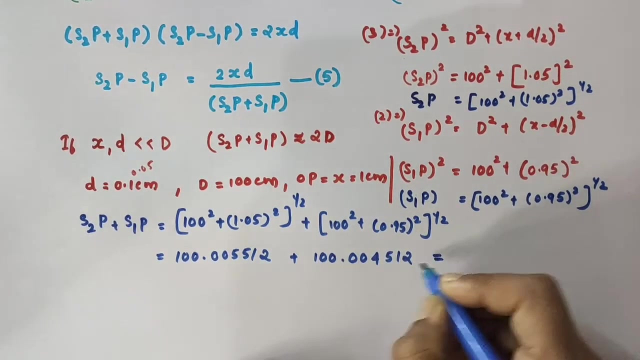 Then, while you are doing this calculation, you will get almost 100.005512 like that. Okay, Okay, so. So, while you are adding these two, you will get almost 200.010024.. So, approximately, you can take S2P plus S1P as 200.01 centimeter. 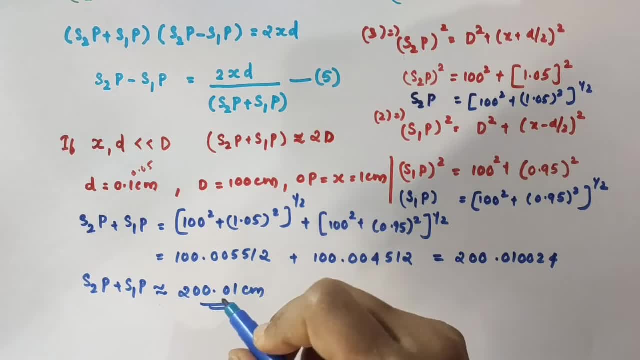 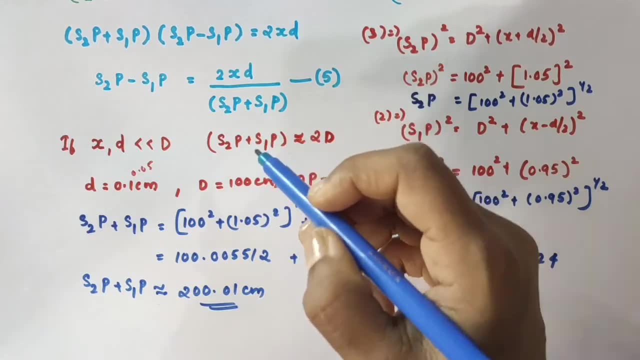 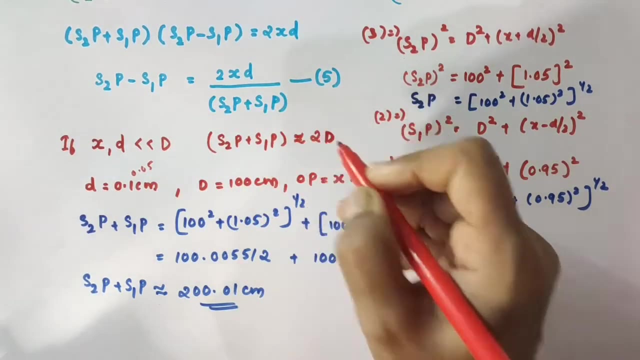 So approximately, we are taking S2P plus S1P as 200.01 centimeter. So this is the. This is the actual value for this denominator S2P plus S1P. Okay, Now, if we replaced this denominator S2P plus S1P by 2D- 2 into capillator D- then that becomes what. 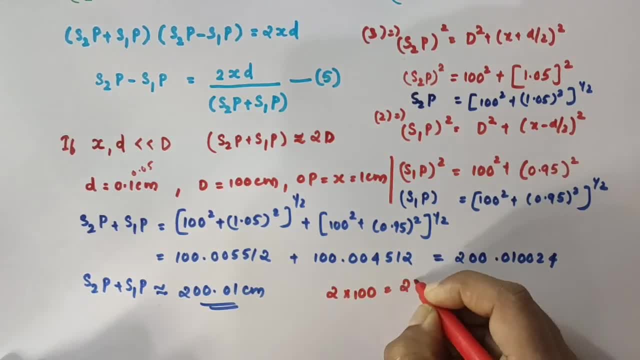 2 into capillator D is 100 centimeter, So this becomes 200 centimeters. So this is the actual value And when we replace this denominator by 2D, we are getting 200 centimeter. See 200.01 centimeter and 200 centimeter. 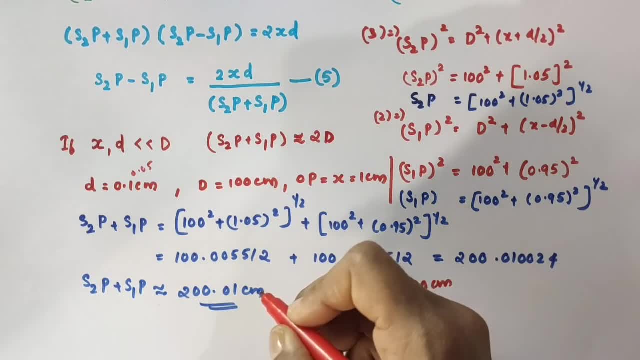 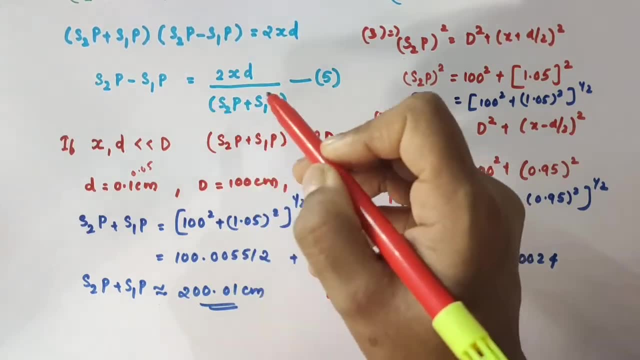 See the The difference is only 0.1 centimeter. Okay, That is not a big difference. actually. Actual value is 200.01 centimeter And when we are replacing this S2P plus S1P by 2D, we are getting 200 centimeter. 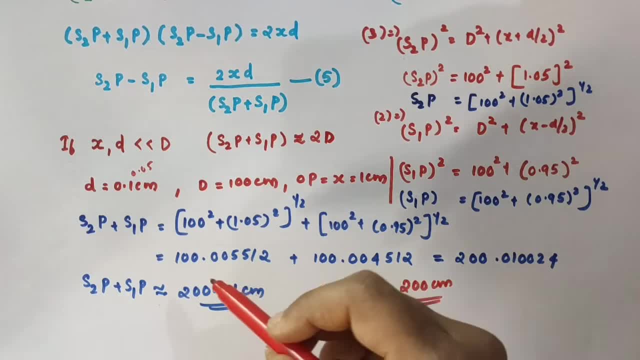 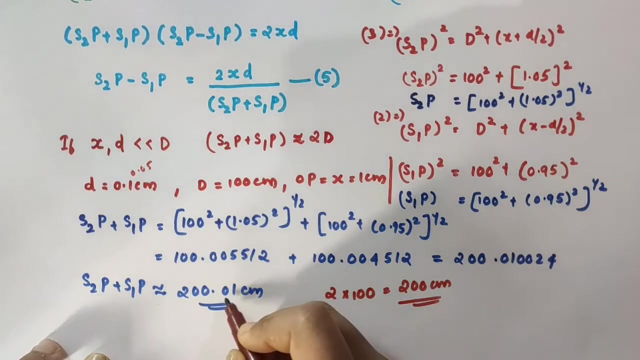 So the difference is only 0.1 centimeter. Actual value is 200.01.. No, So the difference is only 0.01 centimeter. Okay, Now see if I am taking like, If I am taking X, percentage of 200 is 0.01.. 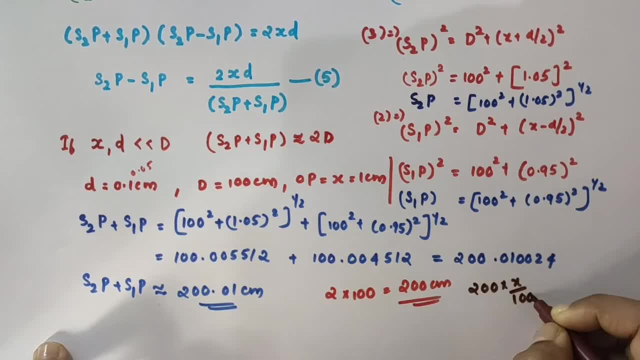 That is, 200 into X by 100 is equal to 0.01.. So X is equal to 0.01.. Cancel no. So 0.01 divided by 2. That becomes 0.005 percent. 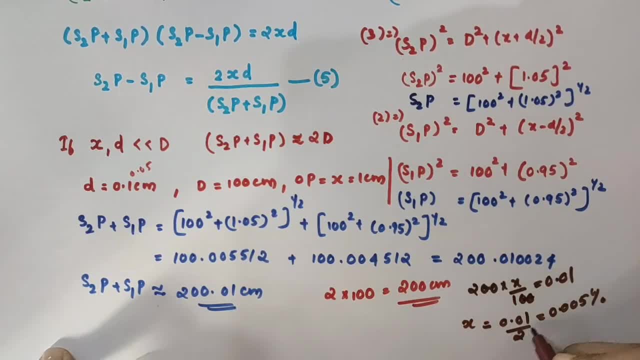 Okay, I am taking X percentage of 200.. So 0.01 is 0.01.. So we are getting XX, 0.005 percent. That is the actual value for S2P plus. S1P is about 200.01 centimeter. 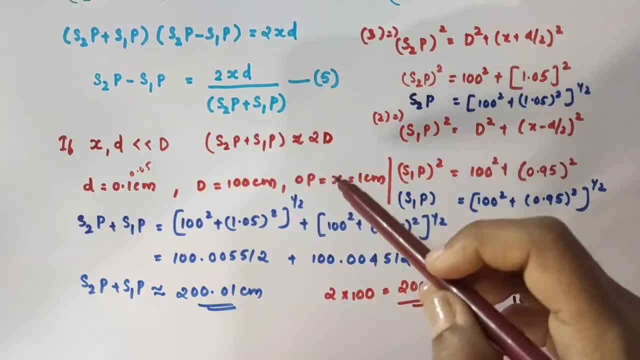 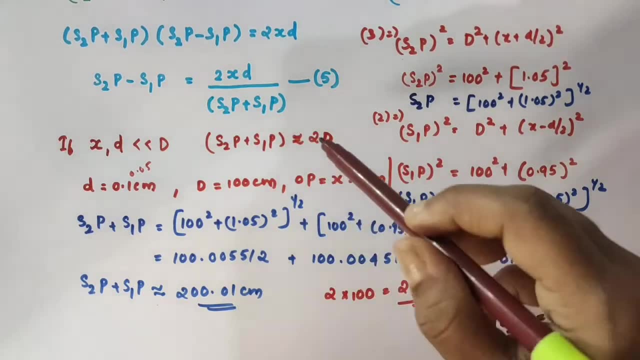 When we replace S2P plus S1P by 2 into capillator D, we get 200 centimeter. That is, if we replace S2P plus S1P by 2D, the error involved is only about 0.005 percent. 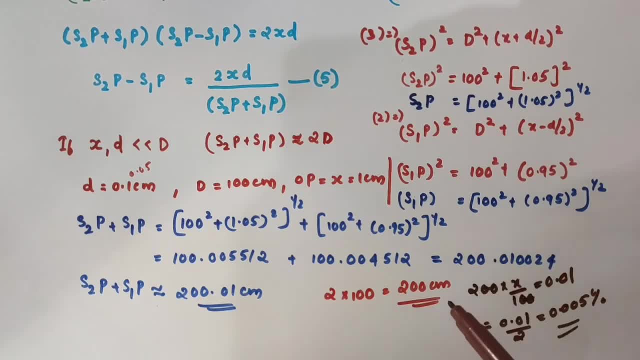 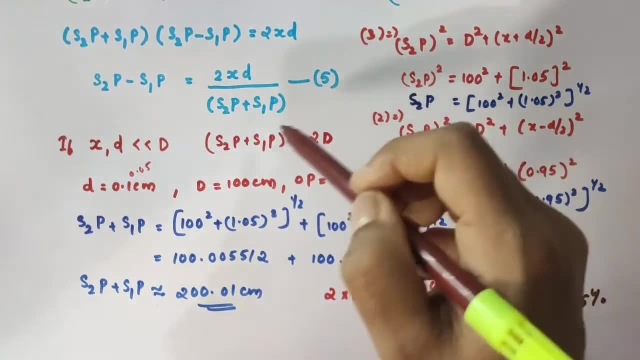 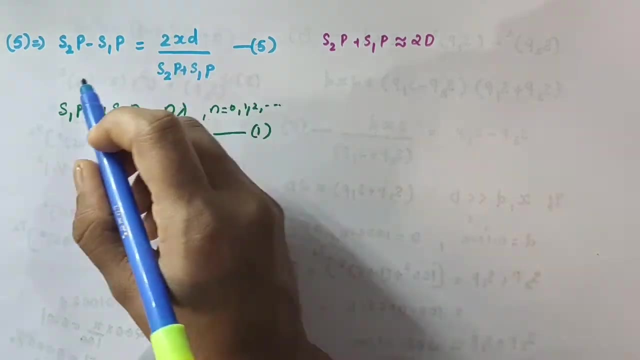 Okay, Okay. Okay, That is only a negligible error is introduced in the result, So it is not that much a big problem of taking this approximation. So we can take this approximation. So in this approximation, equation number 5, which is S2P minus S1P, equal to 2XD divided by S2P plus S1P. 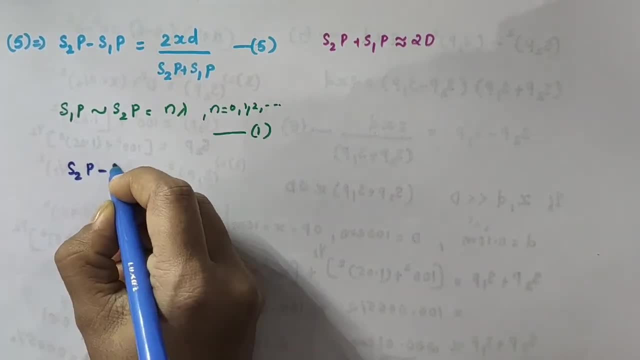 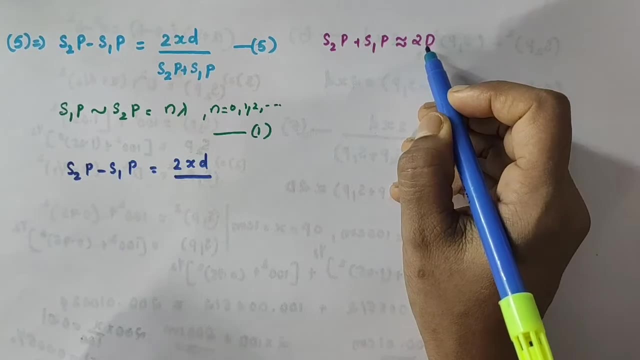 That becomes what S2P minus S1P is equal to 2XD. Divided by S2P plus S1P can be approximated to 2 into capillator D. 2 from the numerator and 2 from the denominator has cancelled. 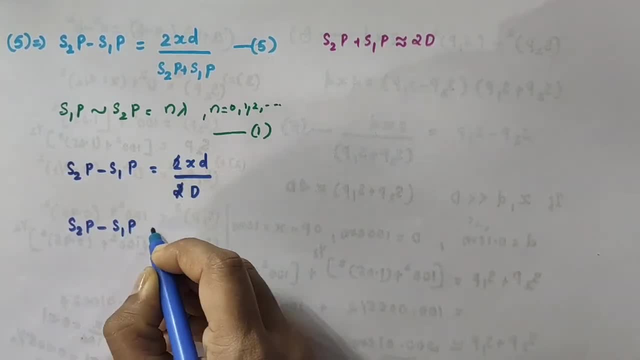 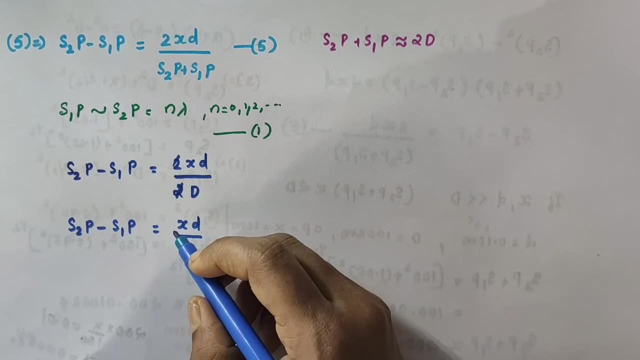 So we can write S2P minus S1P is equal to X into small letter D divided by capillator D, Where X is actually the distance from the origin to the point, distance from the point O to the point, to the arbitrary point P on the screen. 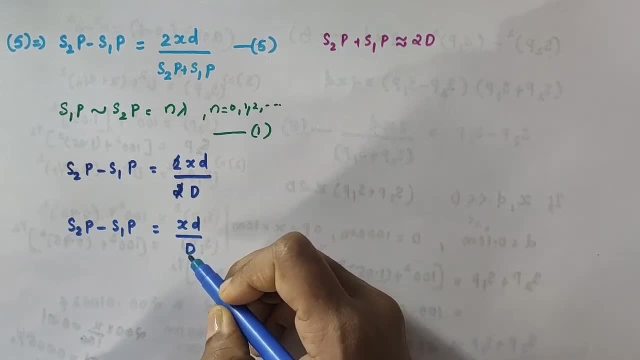 Small letter D is the distance or separation between the two slits, And Capillator D was the distance between the screen and the slit. So we are getting S2P minus S1P is equal to X into D divided by capillator D. 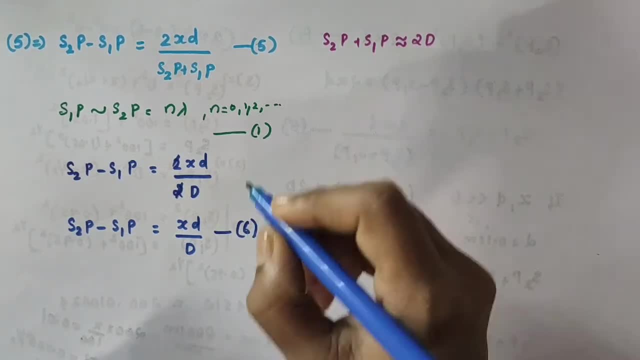 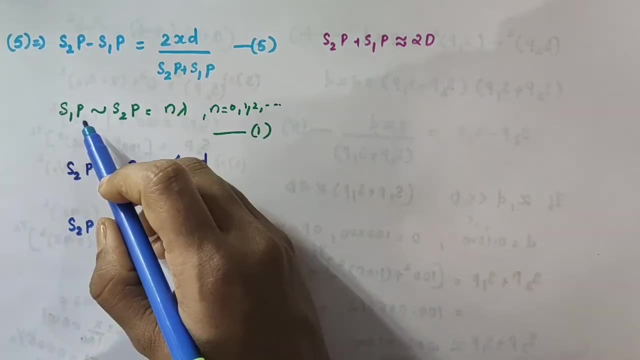 And I am taking this as equation number 6.. And we got equation number 1 like this: S1P- S2P equal to N lambda. This means S1P minus S2P equal to N lambda, or S2P minus S1P equal to N lambda. 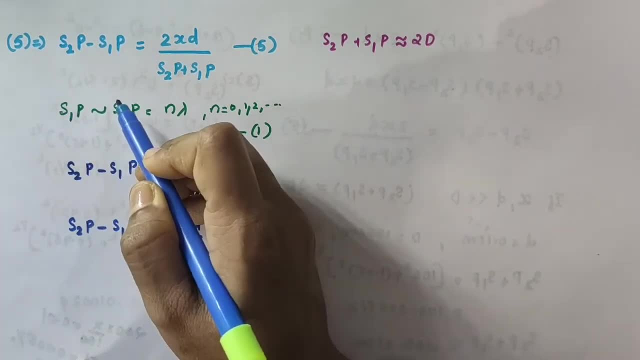 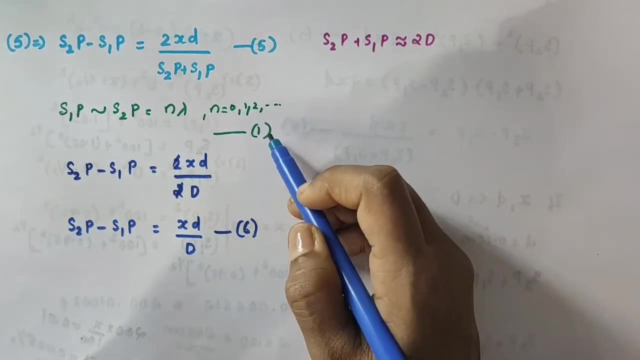 Where this sign actually indicates S1P minus S2P or S2P minus S1P- Both can be taken- Then this N equal to 0,, 1,, 2,, 3, etc. Alright, So I am going to substitute this equation number 1 in equation number. 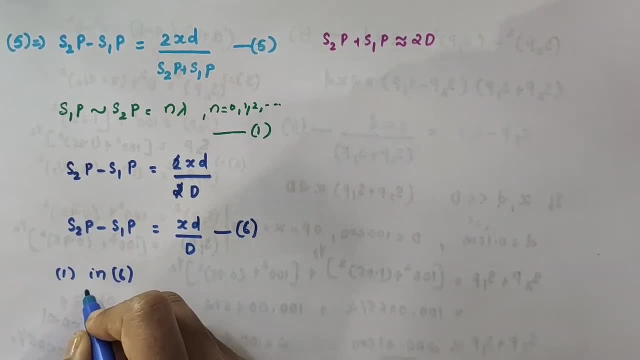 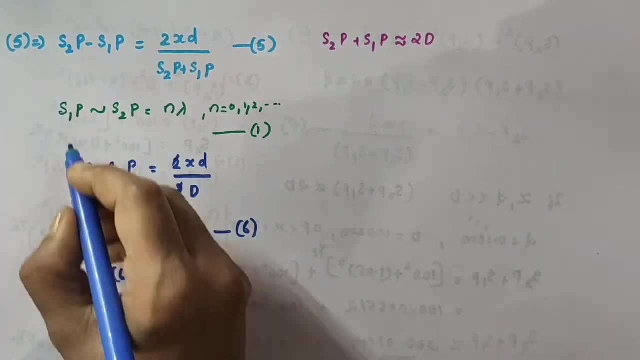 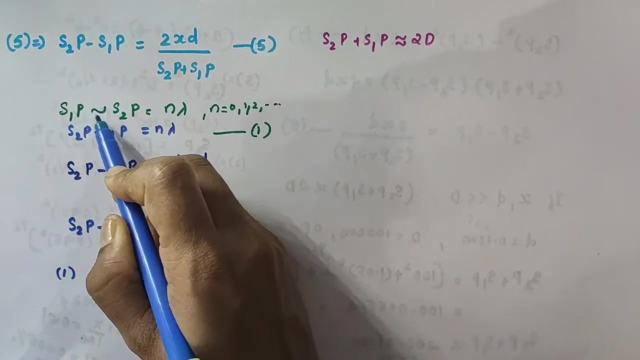 I mean, I am not, I am just going to compare this equation number 1 and equation number 6.. See, this can be written as S2P minus S1P, equal to N lambda, Because S1P this sign actually indicates. 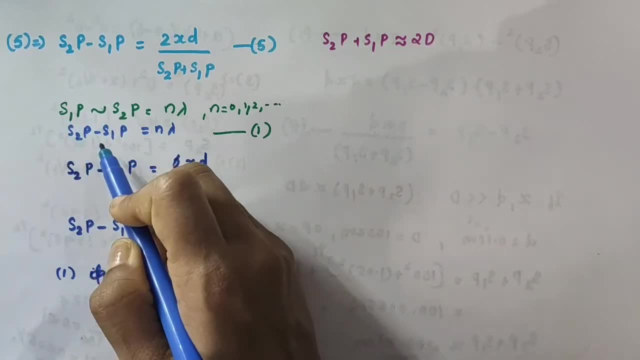 This can be written as S1P minus S2P or S2P minus S1P. So I am writing it as S2P minus S1P, equal to N lambda. So here we have S2P minus S1P, equal to N lambda. 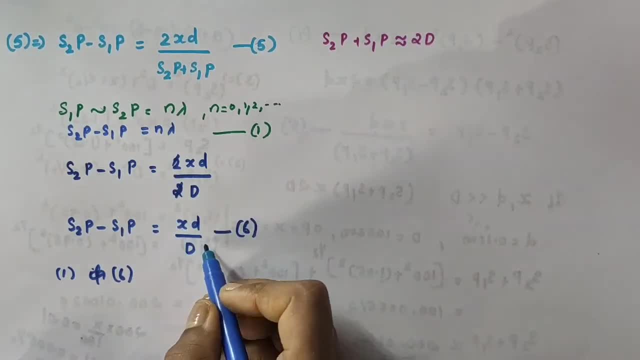 So when we substitute that equation number 1 in equation number 6, we can replace this by N lambda. Okay, So N lambda equal to X into D divided by capital D. Okay, That is, if I am taking See, this can be written as N lambda is equal to X into D divided by capital D. 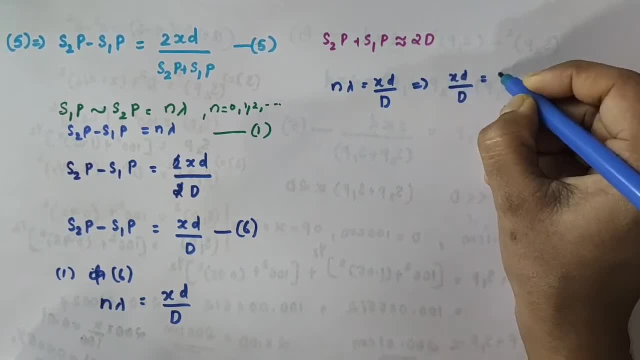 Okay, So this can be written as: N lambda is equal to X into D divided by capital D. Or this can be written as: X D divided by capital D is equal to N lambda. Same equation Next. X is equal to: 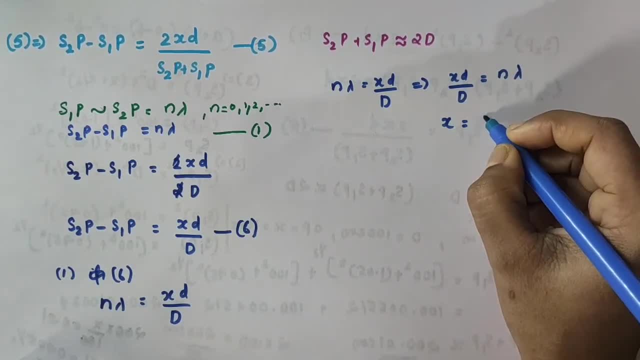 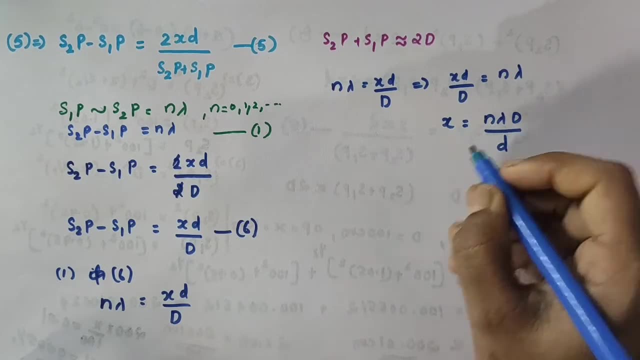 I am taking this D by D to the other side, So this becomes N lambda into capital D divided by small letter D. Okay, Or in general this can be written as X. N is equal to, Because N is here. 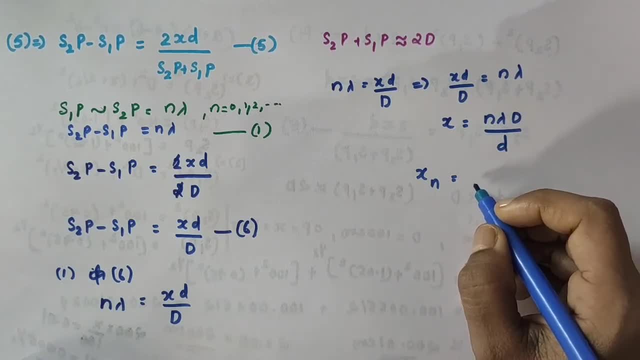 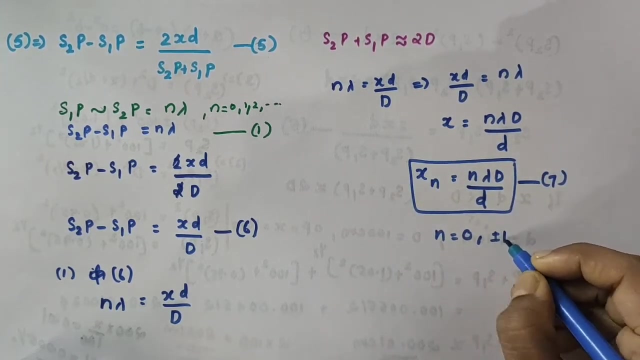 Now this can have different values. So X N is equal to What? N into lambda, into capital D, D divided by small letter D? I am taking this as equation number 7.. Where N equal to 0, plus or minus 1, plus or minus 2,, etc. 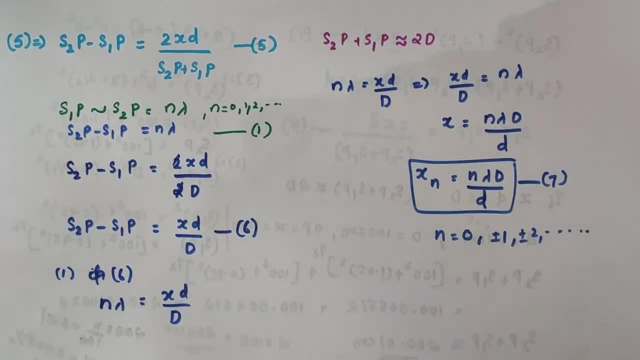 Plus or minus 3, etc. Okay, That is, we will have constructive interference. We will have a constructive interference resulting a bright region. When X, N is equal to N, lambda capital, D by small letter, D Where N equal to 0, plus or minus 1, plus or minus 2, plus or minus 3.. 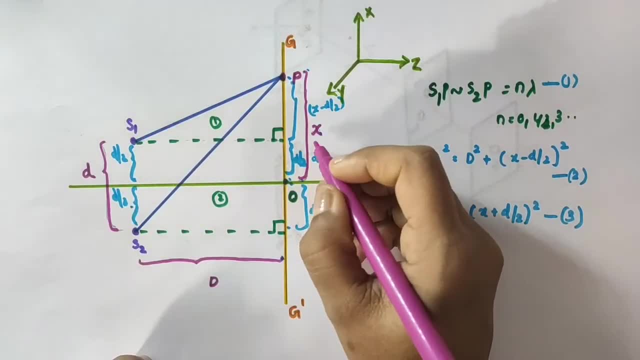 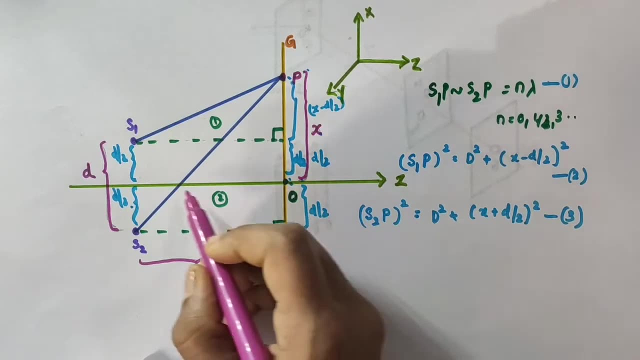 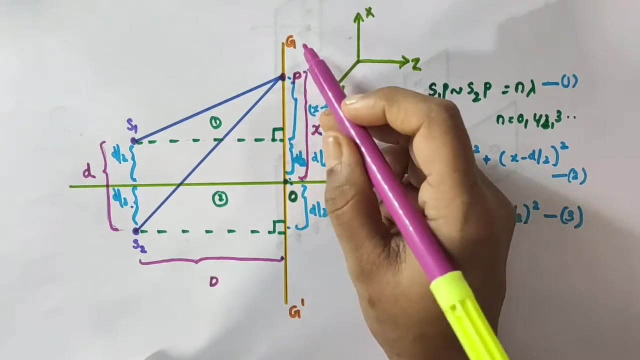 Etc. Now, what is this? X OP equal to X norm. That is here. O is the point on the perpendicular bisector of these two positions of S1 and S2. And P is any arbitrary point chosen on the screen. 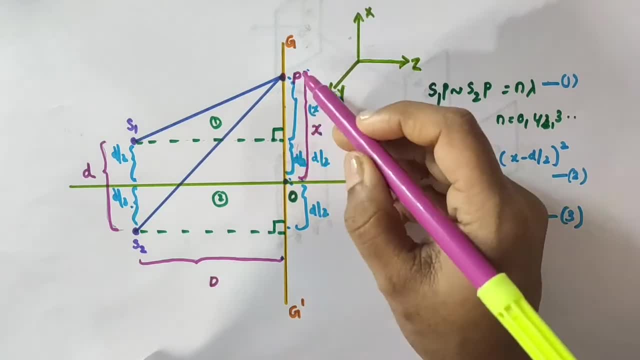 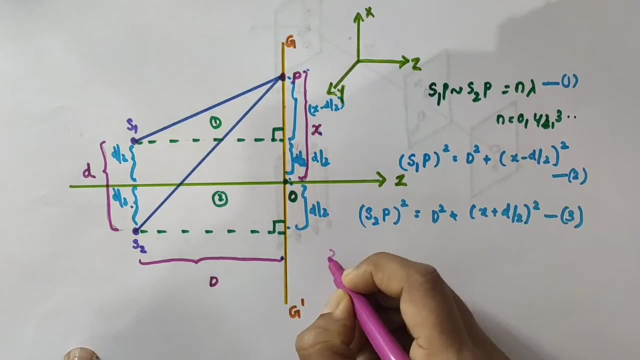 You can take P some way here. P some way here. Okay, OP, is the distance from the point O to the point P. Alright, Now see from equation number 7.. And we got X. N is equal to X. N is equal to N. lambda capital letter D by small letter D. 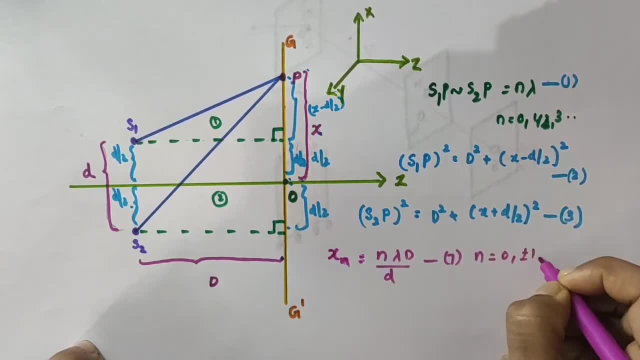 This was equation number 7.. Where N equal to 0, plus or minus 1, plus or minus 2, plus or minus 3, etc. Okay, Now, when N equal to 0, small letter: N equal to 0.. 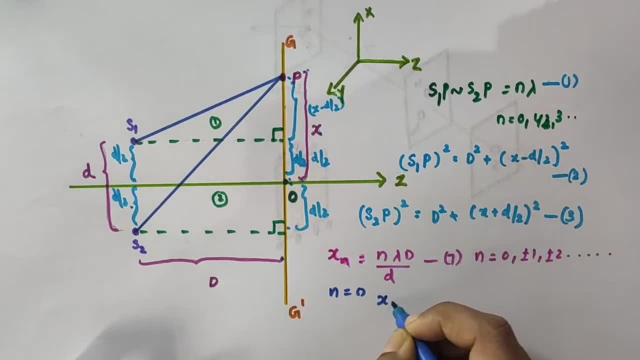 This equation becomes what X is equal to actually X 0. here, X 0 is equal to N 0.. No 0 into any value will give us 0.. Okay, That is X equal to 0.. 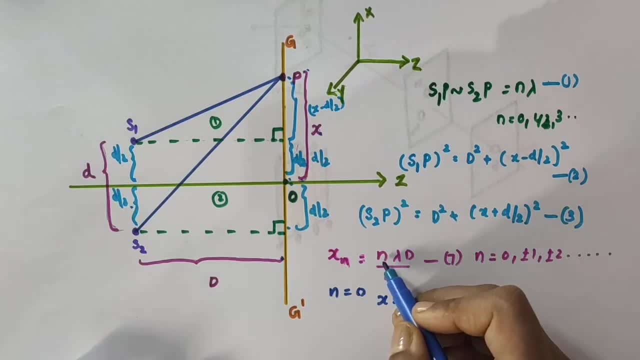 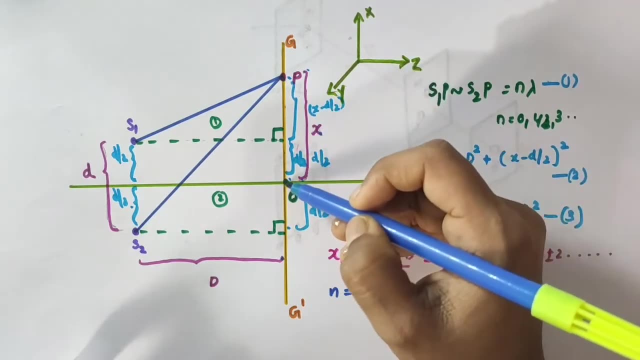 When N equal to 0, X equal to 0. Okay, That is, there is no distance between O and P. X equal to 0 means X is actually the distance from the point O to the point P. X equal to 0 means what? 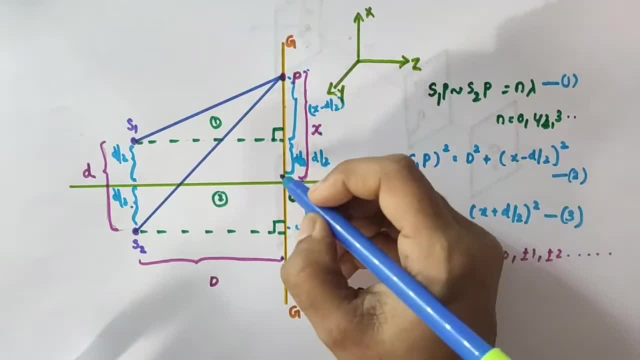 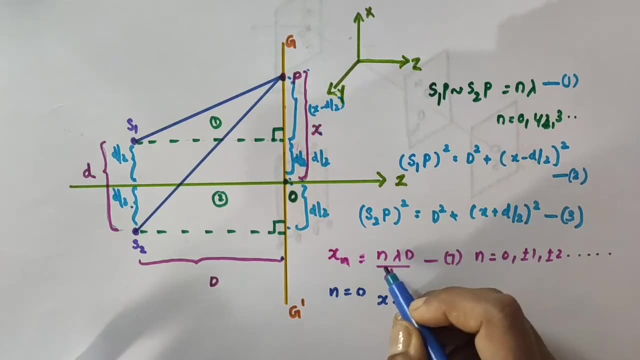 There is no distance between P and O. That means P is here itself, at the point O. Okay, So at the point O. this is actually the condition For the constitutive interference. Now, so when N equal to 0, X equal to 0.. 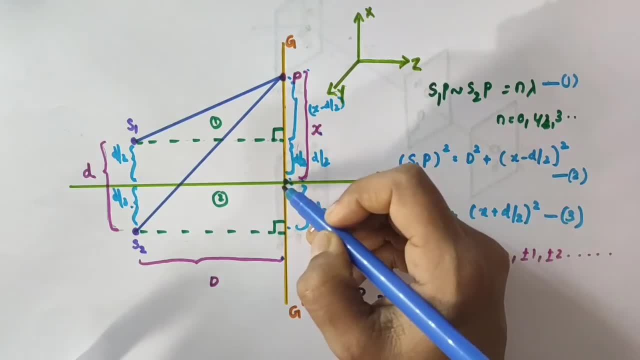 X equal to 0 means this point P is somewhere here at the point O itself. So at the point O constitutive interference take place. Okay, Constitutive interference takes place here, at this point O, And we will get maximum intensity of light. 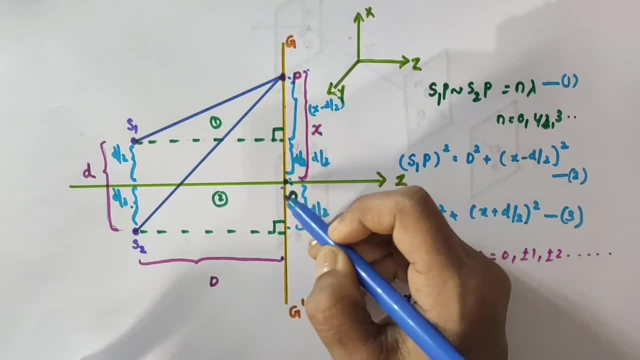 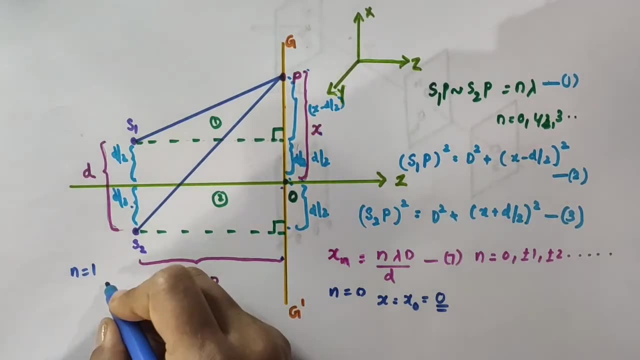 That is a bright band of light here. at the point O: Alright, Now, when N equal to 1.. Okay, When N equal to, When N equal to 1, this X actually becomes XN. now, That is, X1 is equal to 1. into lambda capilator D, divided by small letter D. 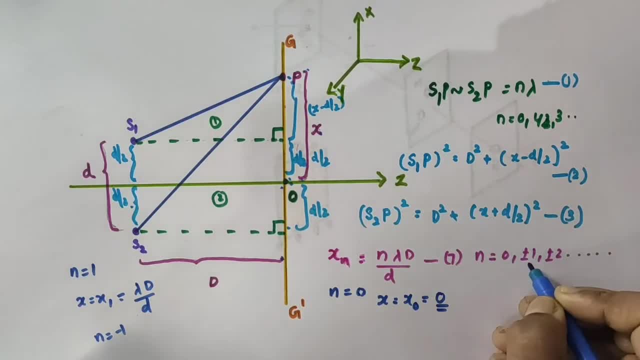 Okay, This N can be minus 1 to N equal to plus or minus 1.. So when N equal to minus 1, X minus 1 is equal to minus lambda capilator D by small letter D. Okay, Similarly, that is X equal to lambda D by capilator D. 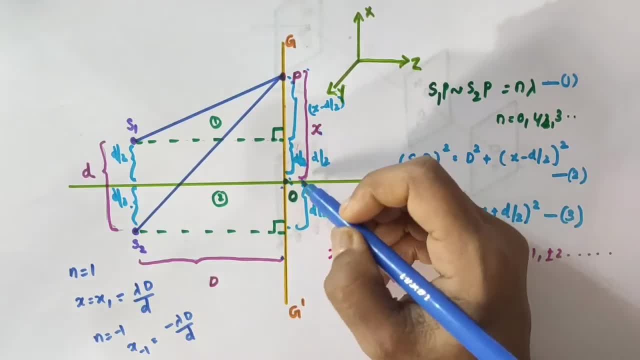 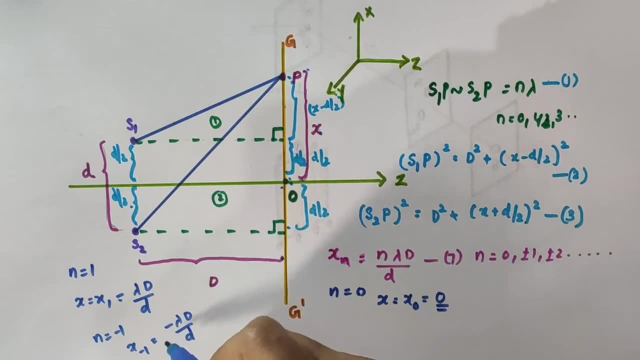 This means above the origin, I mean above the point O, A bright band from the point O That is above O, That is from the central maximum. Okay, Then N equal to minus 1.. We are getting minus lambda D by cap. 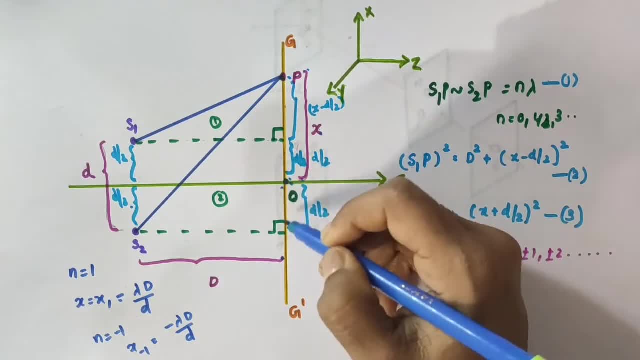 Small letter D, So minus lambda D. by D means below the, I mean below the point O. Okay, We will get a bright band above the point O as well as below the point O. Similarly, for N equal to plus or minus 2, we will get X. plus or minus 2 is equal to. 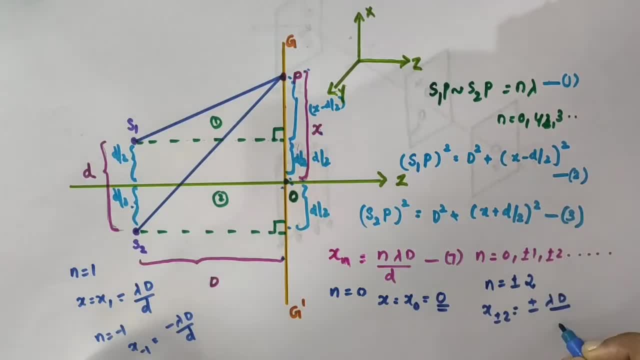 Plus or minus lambda capilator D. by I mean plus or minus 2 lambda capilator D by small letter D, That is at the point X equal to 0, X equal to lambda D by D, minus lambda D by D, X equal to plus 2 lambda D by D, X equal to minus 2 lambda D by D, etc. 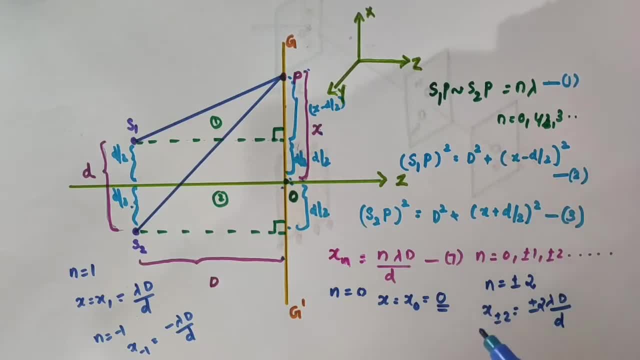 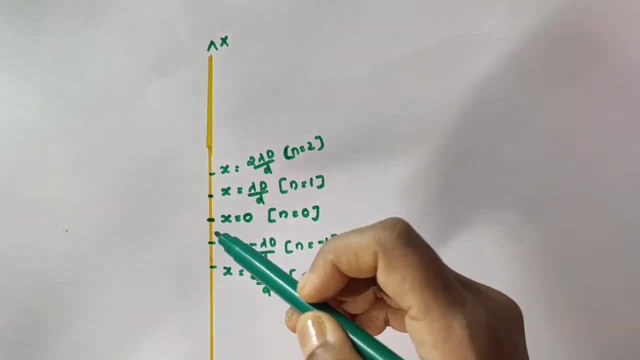 At all these points we will get bright bands of light. Okay, So at X equal to 0, that is the central maximum, X equal to 0 and X equal to lambda D by D, X equal to minus lambda capilator, D by small letter D, which is corresponding to that N equal to minus 1 value. 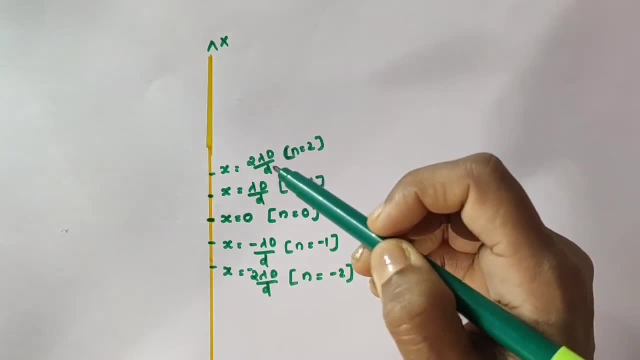 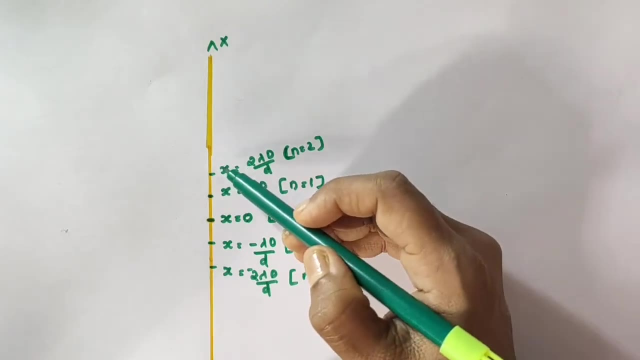 Then N equal to 2, X equal to 2 lambda capilator D by small letter D. And for N equal to minus 2, X is equal to minus 2 lambda capilator D by small letter D. So at all these points on the screen, the screen is actually taken along the X axis. 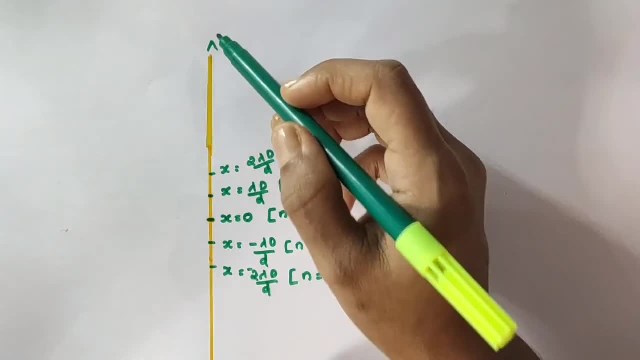 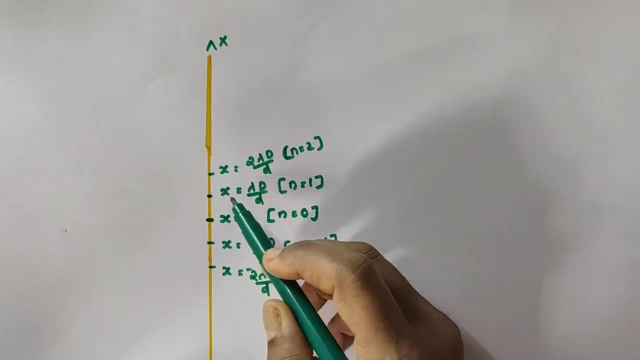 X axis is actually taken like this here. So let's At all points on the X axis, at all points on the screen, at all these points, okay, X equal to 0, X equal to lambda D by D, 2 lambda D by D, then minus lambda D by D. 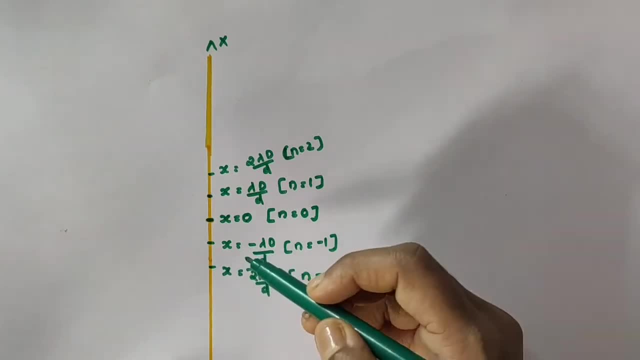 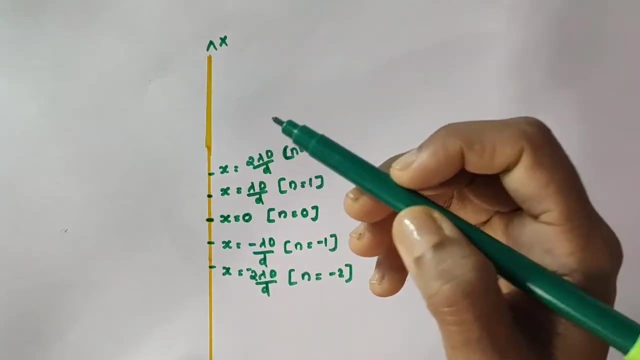 At all these points on the screen, constructive interference will take place and we will get maximum intensity, Okay. So at all these points- there will be so many other points, because N can have 0, plus or minus 1, plus or minus, 2, plus or minus 3,, etc. 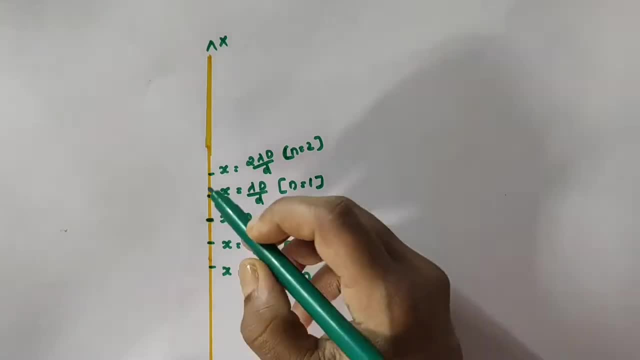 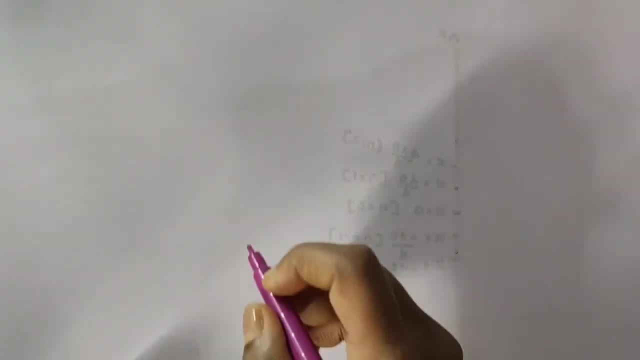 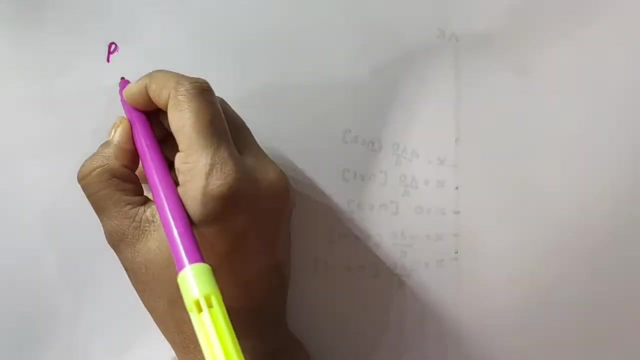 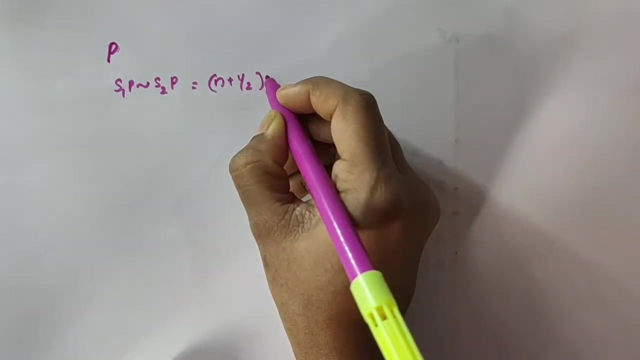 Here we have considered only 0, plus or minus 1 and plus or minus 2.. So, corresponding to all these points, we will get Bright bands of light on the screen. In our previous video we have seen that at any arbitrary point P- okay, at any arbitrary point P- the condition for destructive interference is S1P. S2P is equal to N plus half into lambda. 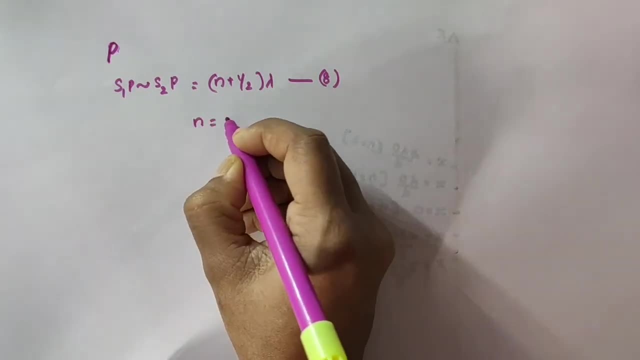 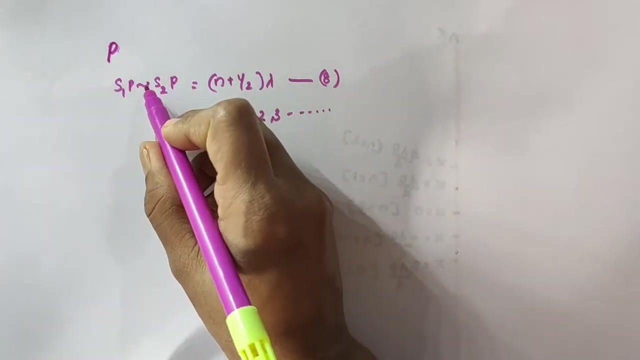 I am taking this as equation number 8.. Where N equal to 0,, 1,, 2,, 3, etc. Okay, S1P. this symbol actually indicates that this can be written as S1P minus S2P or S2P minus S1P. 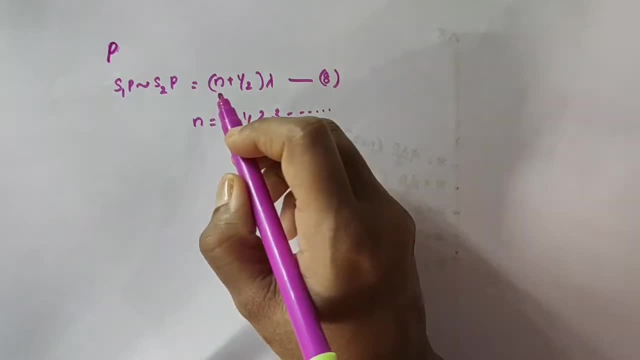 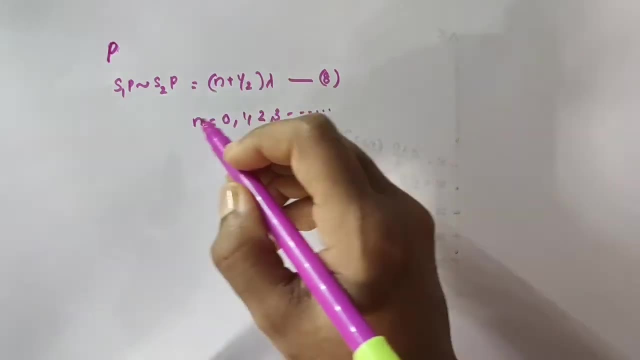 If that is equal to, that is actually the path difference. no, If that is equal to N plus half into lambda, where N equal to 0,, 1,, 2, 3, etc. we can say that this is actually the condition for the destructive interference. 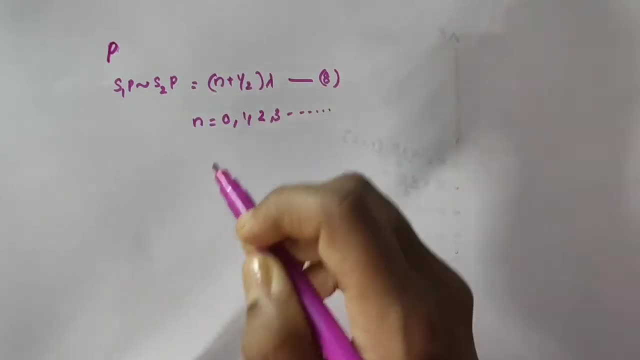 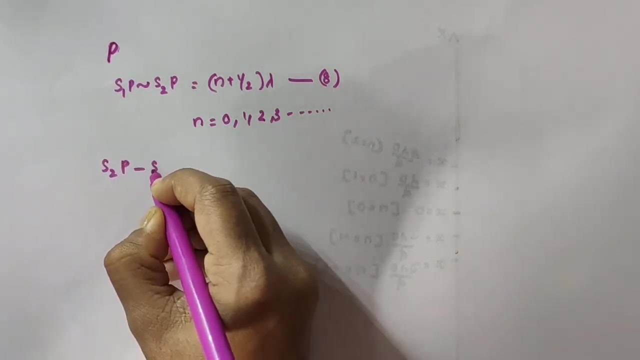 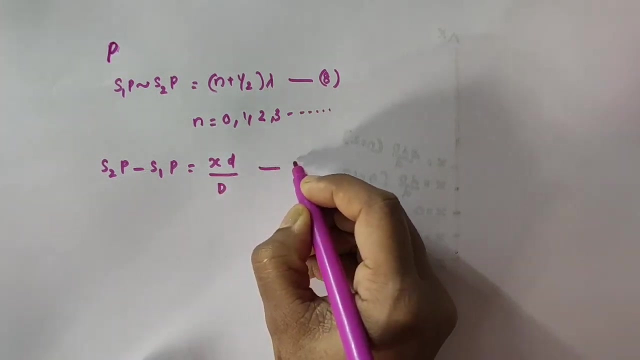 So cannot constructive. this is actually the condition for the destructive interference. Okay, Then from equation number 6, we have: S2P minus S1P is equal to X into small letter D divided by capital letter D. This was actually equation number 6.. 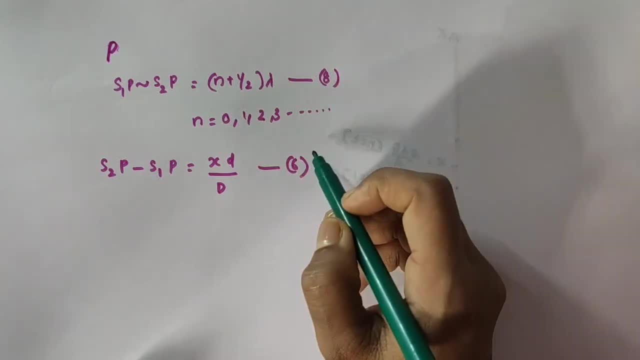 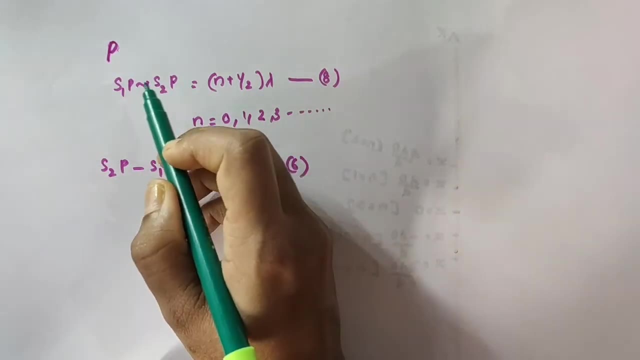 Now from this equation number 8 and equation number 6, see this is S2P minus S1P is equal to XD by D. This is S1P minus S2P, or this can be written as S2P minus S1D. 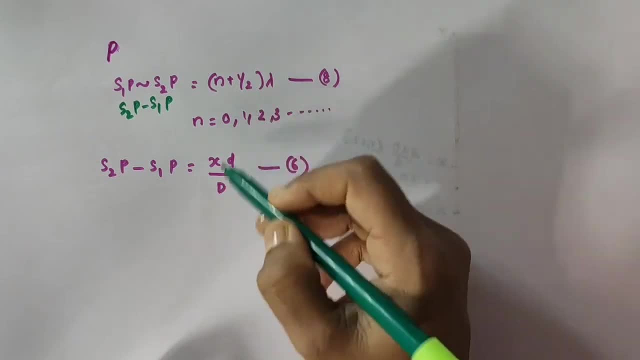 S2P minus S1P is equal to N plus half into lambda. So when we compare these two we can write: these two are the same. no, I mean left hand side of these two equations are the same, no. 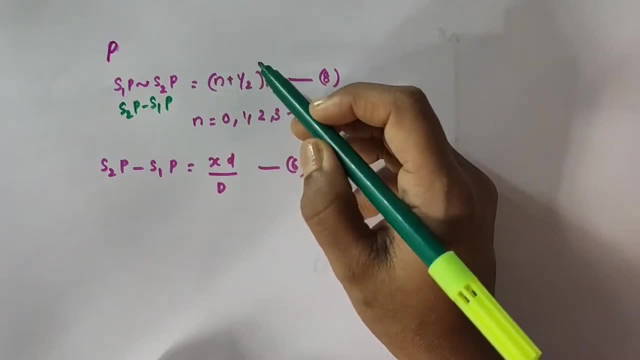 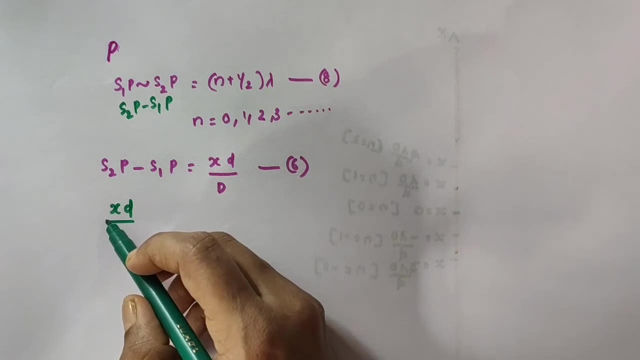 S2P minus S1P, S2P minus S1P, So we can equate their right hand sides, That is, we can write X into small letter D divided by capital letter D. Okay, Where X is the distance from the point O to the arbitrary point P on the screen. 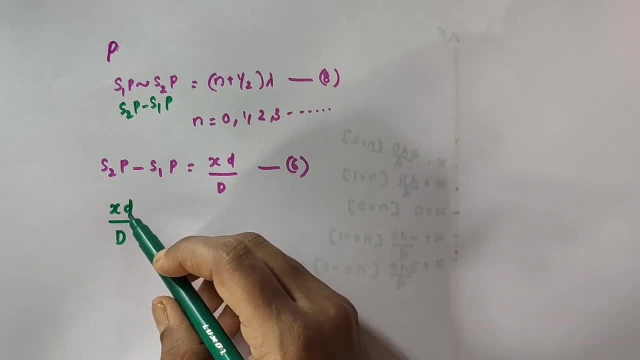 Small letter D is the distance of separation between the two slits or two holes, S1 and S2.. Then capital letter D is actually the distance from S1 and S2 to the screen. So this is equal to what N plus half into lambda. 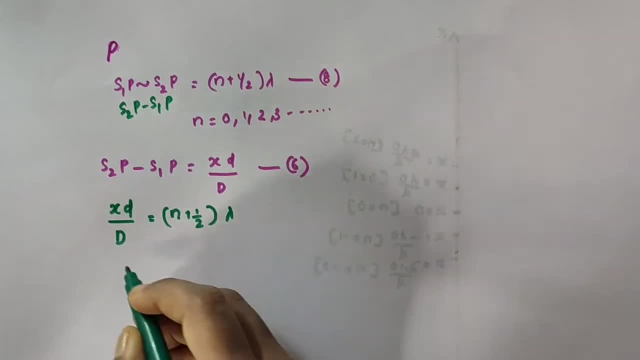 Okay, Next I am taking this D by D to this side, So this becomes: X is equal to N plus half into lambda. Capital letter D goes to the numerator and small letter D comes to the denominator. Or in general we can write it as XN equal to, because N can vary no. 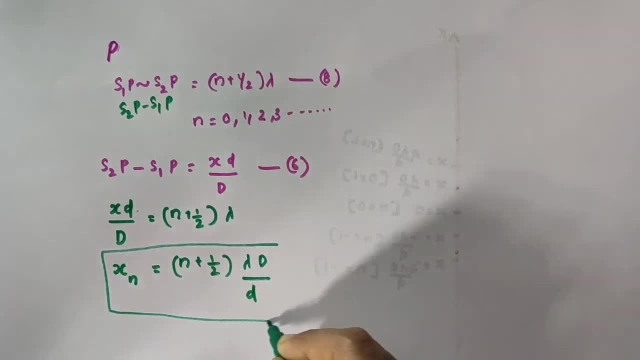 So in general we can write: XN is equal to N plus half into lambda capital letter D by small letter D, where N equal to 0, plus or minus 1,, plus or minus 2, plus or minus 3,, etc. 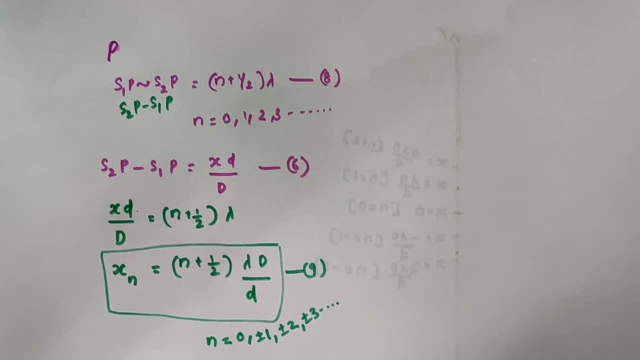 And I am taking this as equation number 9.. That is, we will have destructive interference which results a dark region when XN is equal to N plus half into lambda capital letter D, Capital letter D by small letter D, where N equal to 0,, plus or minus 1, plus or minus 2,, plus or minus 3,, etc. 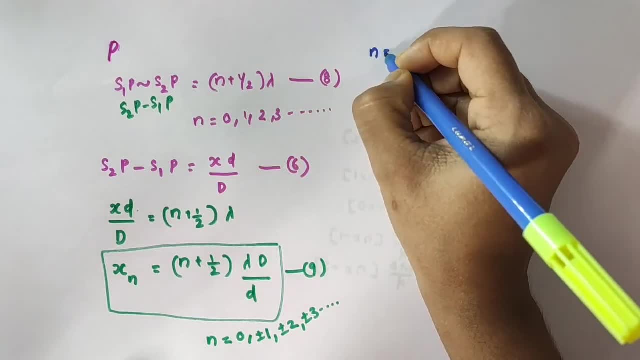 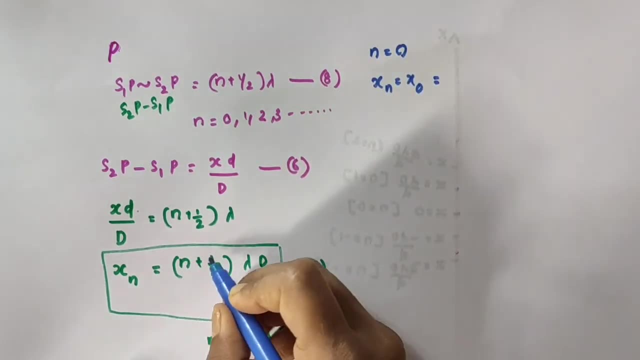 Now, when N equal to 0, I am just substituting N as 0. Then XN, that becomes X0, which is equal to N, equal to 0, no, So 0 plus half, half, Half into lambda capital letter D by small letter D. 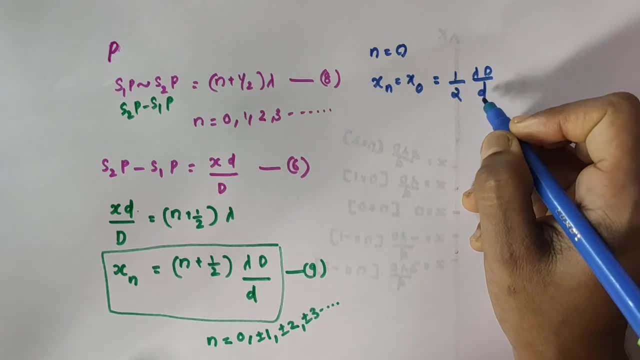 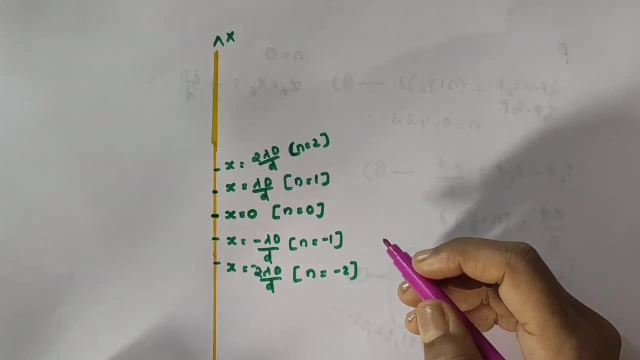 Okay, So at X equal to half lambda capital, Capital letter D by small letter D, we will have the minimum intensity of light or we will have a dark band of light. See in this figure that is. this is actually the screen. 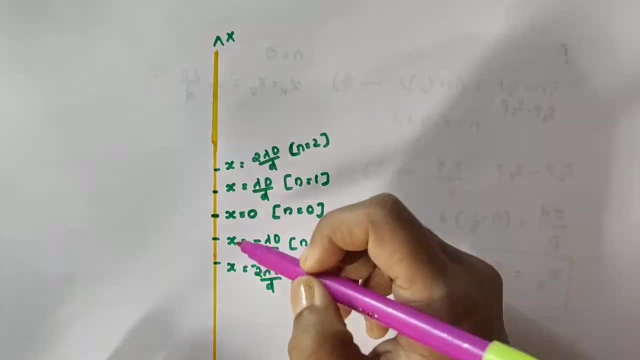 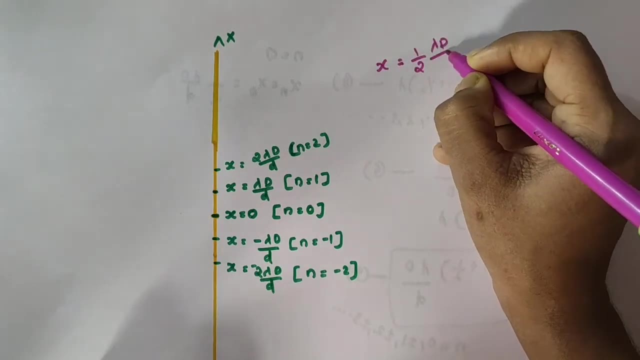 and these are actually the points on the screen- which corresponds to bright bands of light. So we got, when X equal to half into lambda capital letter D. by small letter D, we will have the dark band of light, We will have destructive interference and corresponding to that, 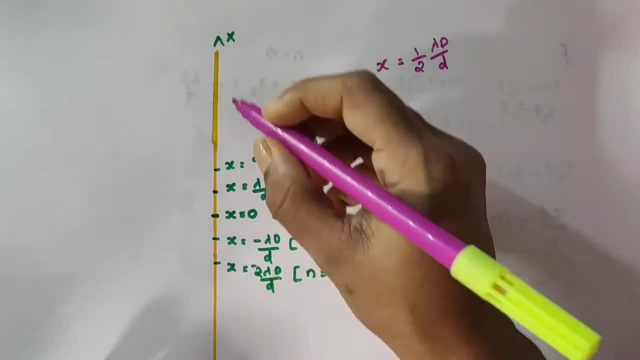 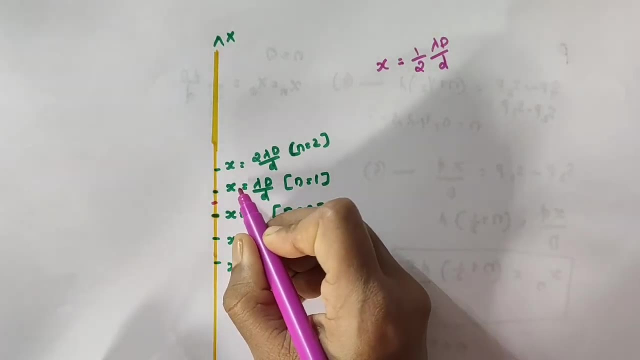 we will get minimum intensity of light and we will have a dark band. So we will have the dark band of light on the screen. So half lambda capital letter D by small letter D light somewhere here. no, Okay, this is X equal to 0.. 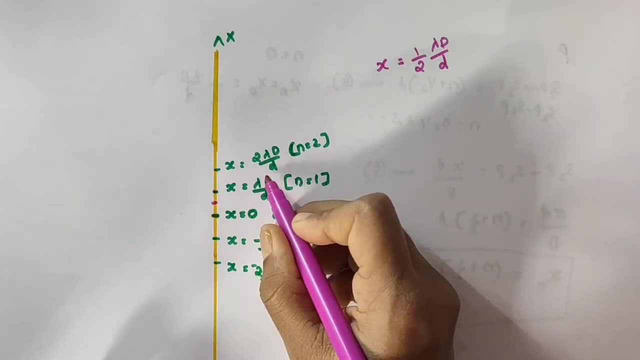 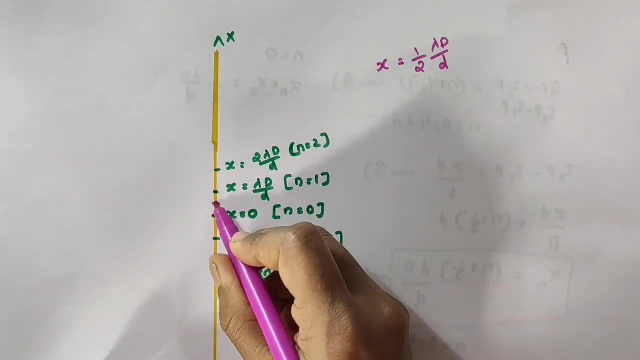 This is. I mean, this is 0,. this is lambda D by D. So half lambda D by D will be in the middle of these two. So at this particular point we will have minimum intensity of light and we will have a dark band of light. 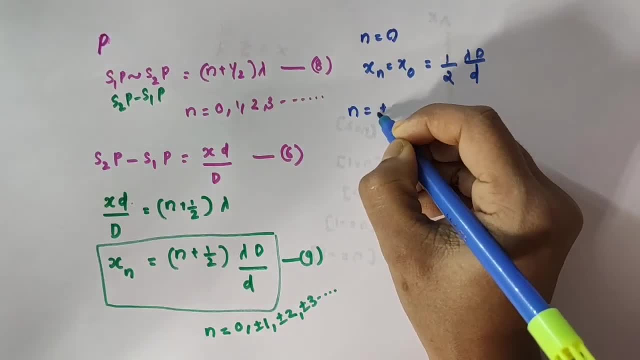 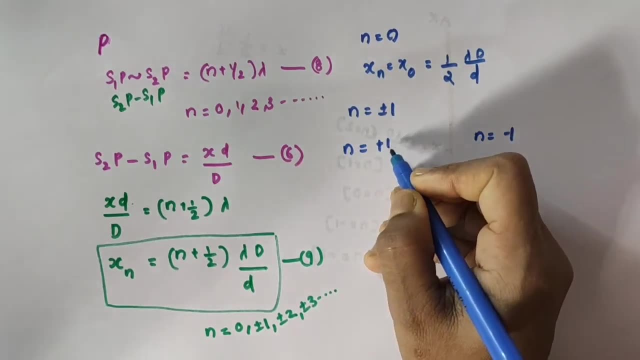 Next, I am taking N as plus or minus 1.. N equal to plus or minus 1.. That is, we can take N as plus 1.. We can take N as minus 1.. So when I am taking N as plus 1,, 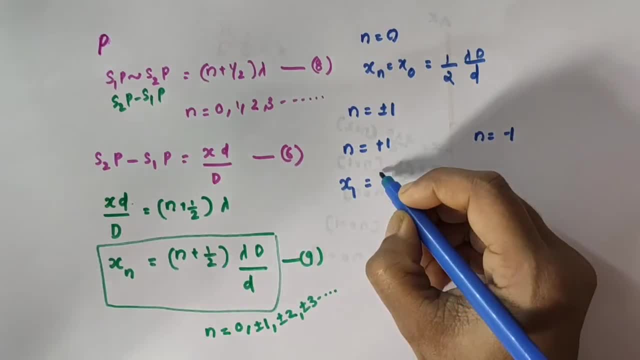 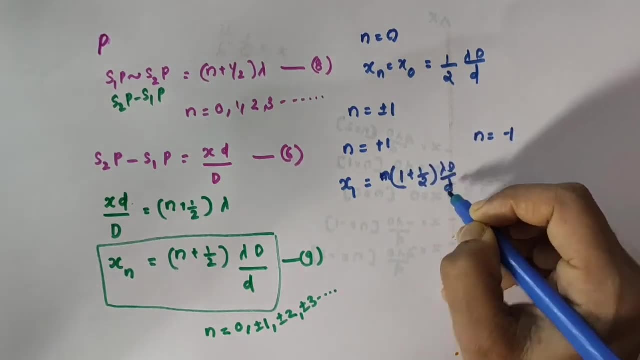 XN becomes X1, which is equal to N plus N is 1, no. So 1 plus half into lambda capital letter D by small letter D. 1 plus half is actually 3 by 2.. 3 by 2- lambda capital letter D by small letter D. 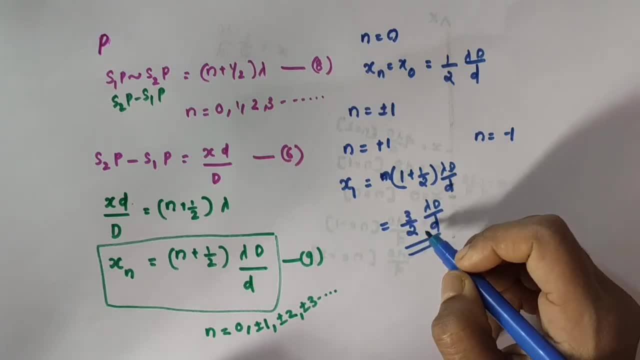 So, corresponding to 3 by 2 lambda capital letter D by small letter D, we will have a destructive interference and, corresponding to that, we will have a dark band of light. See this: 3 by 2 lambda capital letter D by small letter D. 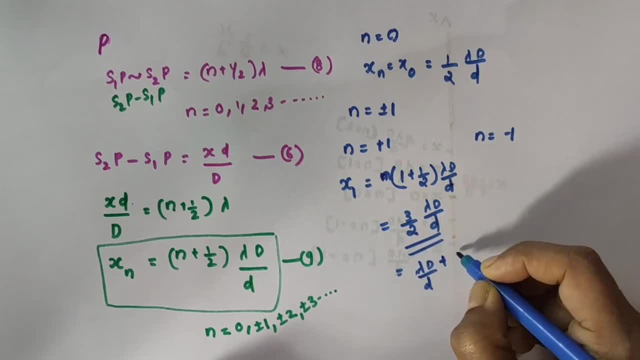 this is actually what: Lambda capital letter D by D plus half into lambda capital letter D by D. Okay, lambda capital letter D by D plus half into lambda capital letter D by D, that is actually 3 by 2. lambda capital letter D by D. 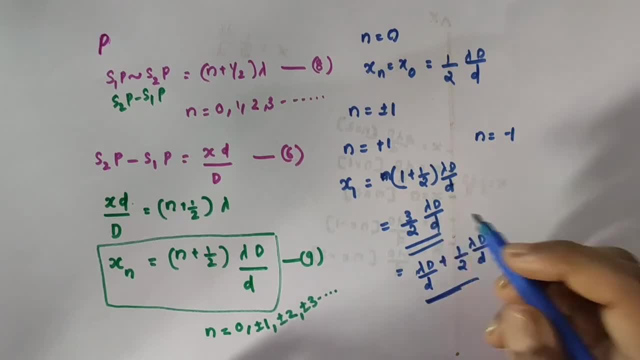 So, corresponding to this, we will have destructive interference. Okay, similarly, when we consider N as minus 1, XN becomes X minus 1, which is equal to N. So 1 plus half, that is minus 1 plus half, into lambda capital letter D by small letter D. 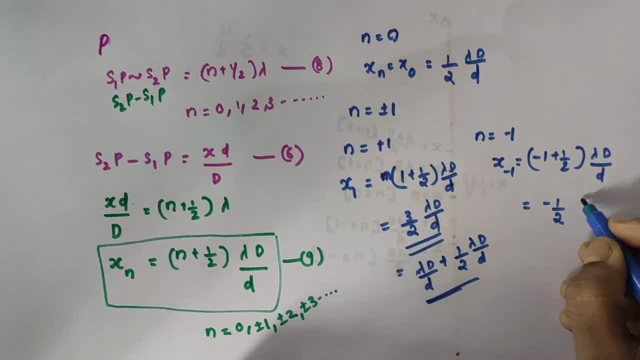 Okay, minus 1 plus half will give you minus half. then lambda capital letter D by small letter D. So corresponding to minus half into lambda capital letter D by small letter D, we will have destructive interference of light and we will have a dark band of light on the screen. 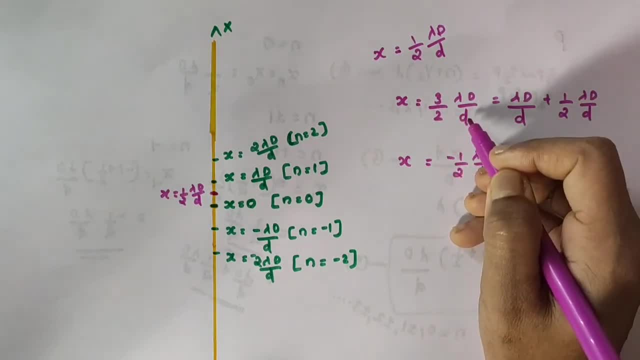 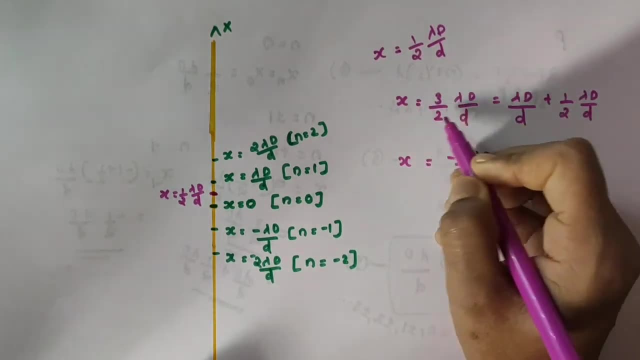 So see, when X equal to 3 by 2 lambda capital letter D by D, that can be written as lambda capital letter D by small letter D plus half into lambda capital letter D by small letter D, Corresponding to this point on the screen. 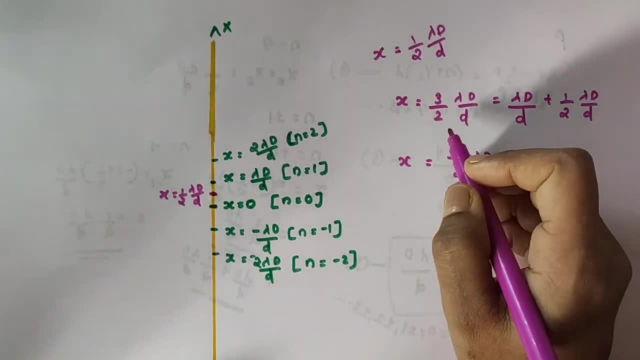 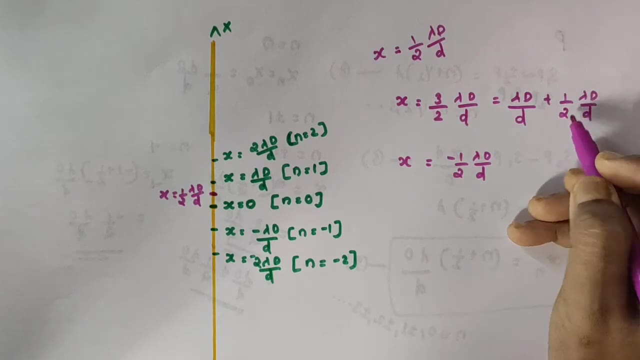 we will have destructive interference and we will get a dark band of light. So see here 3 by 2 lambda, I mean 3 by 2 lambda D by D, that is lambda D by D plus half lambda D by D. no, 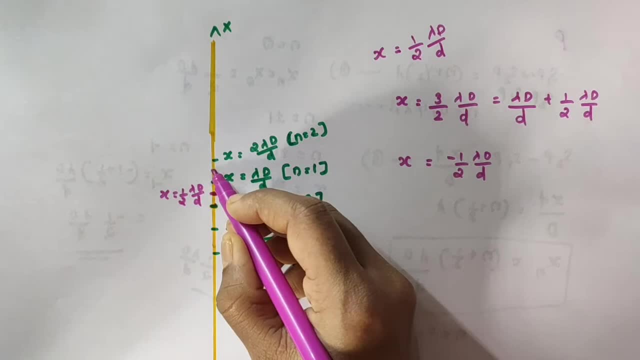 So lambda D by D is half lambda D by D, that is from here to here. that will be my word. 3 by 2. lambda capital letter D by small letter D. So at this point destructive interference is taking place and we will have a dark band of light. 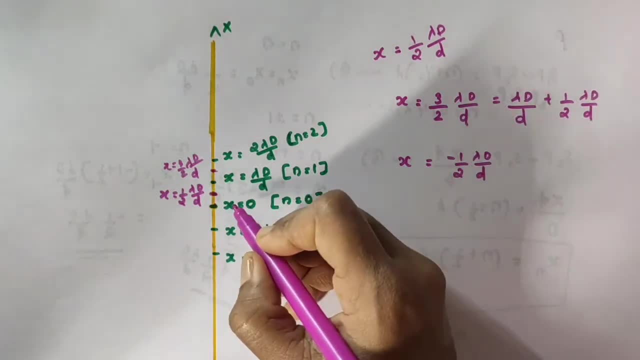 Similarly, when X equal to minus half into lambda capital letter, D by D, See this is X equal to 0, point where we are getting the central maximum and above that point we are taking the positive values and below that point we are taking the negative values. 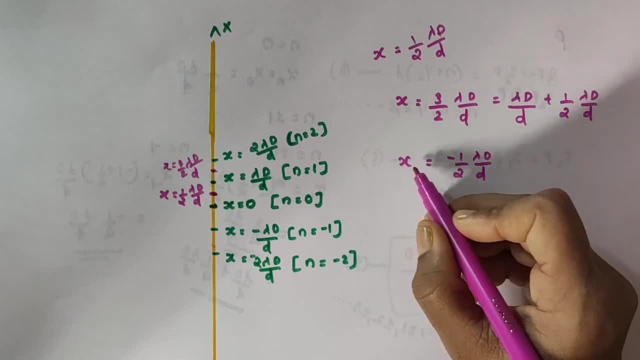 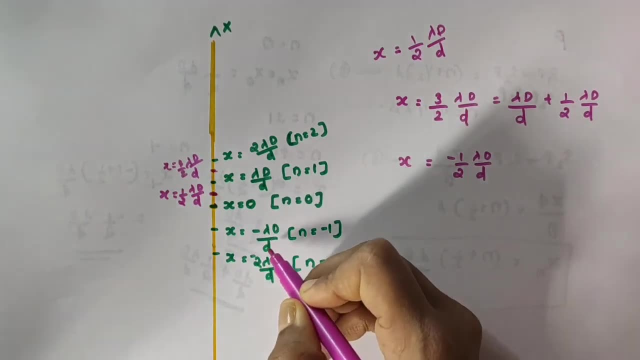 Okay, just like positive X axis, negative X axis, like that. So corresponding to X equal to minus half into lambda capital letter D by small letter D, this is X equal to 0,. this is X equal to minus half lambda D by D.